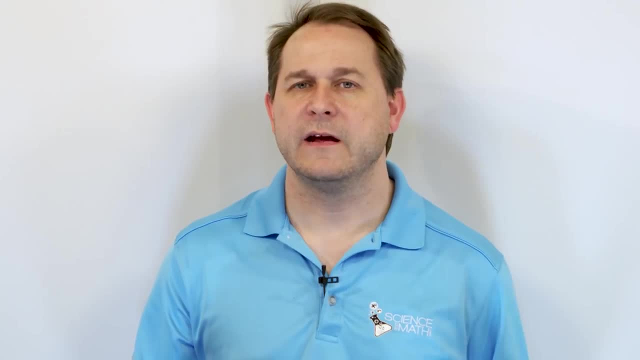 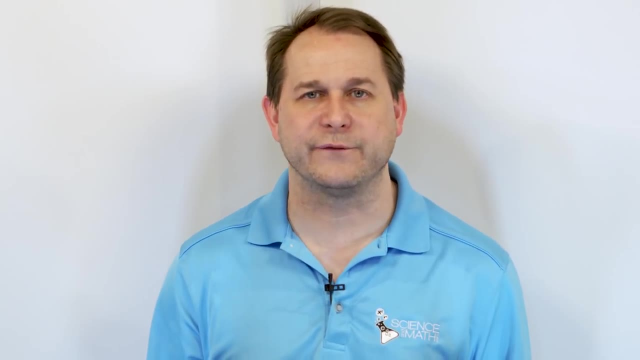 Then we talked about special cases. We talked about those for the last couple of lessons: difference of two squares, perfect square, trinomials, where we can't really pull anything out. but we know they're special cases, so we can write the factor form right away. Here we're going. 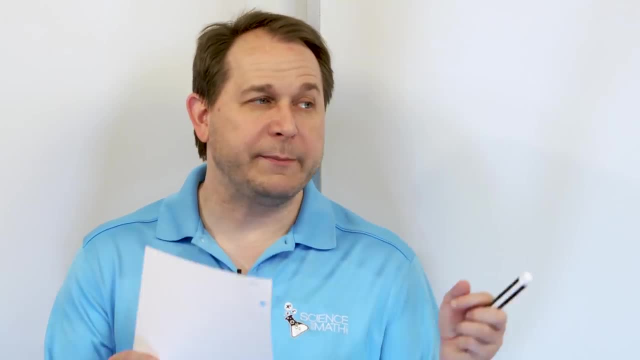 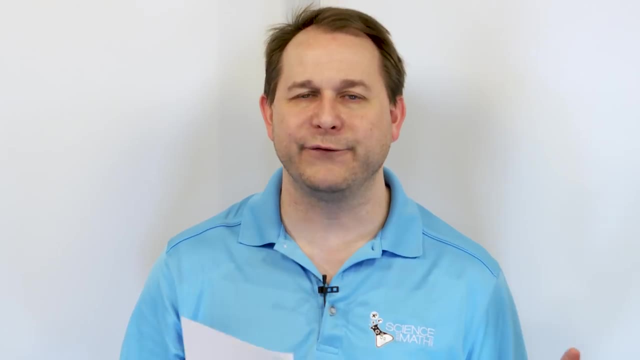 to talk about factoring by grouping. What it basically means is we're going to be looking for common things to pull out, just like before, but it's going to require a little more work to put everything in the correct form in order to pull the proper thing out. It just means we have 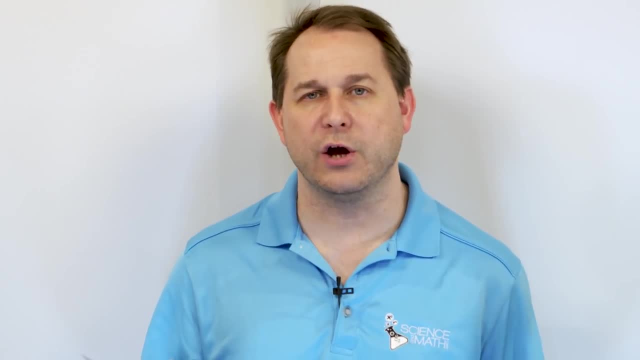 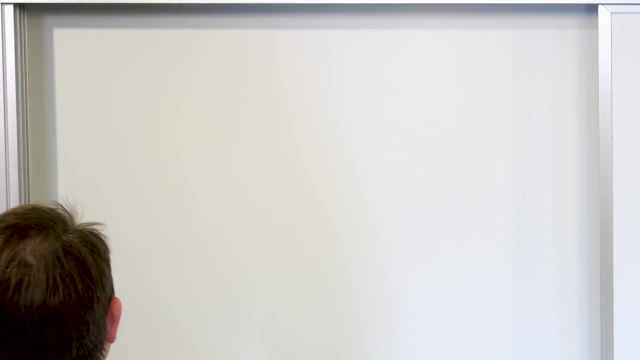 to be a little more creative in what we look for. that happens to be common among all of the terms. To kick us all off, I want to start with something that's very, very simple, that I know that you all understand. What if I give you the expression x times y plus? 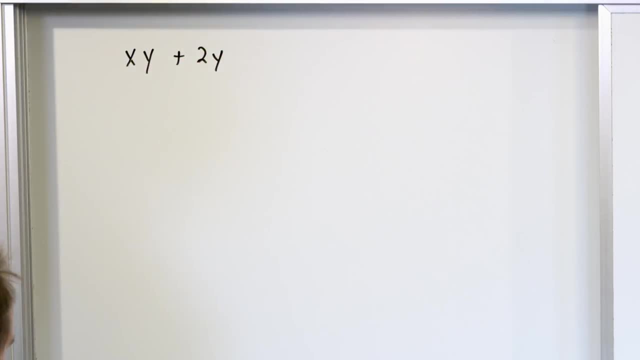 two times y and I say: factor that. The first thing you do is you say: well, I look for what's common. There's an x, but there's no x there, so that can't be common. Here's a two, but there's. 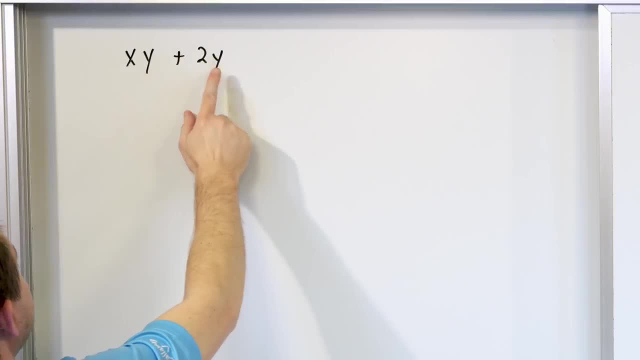 no two there, so that can't be common. Oh, look, here There's a y and there's a y. Y is common, so I can do that right. What I'll do is I'll then say this is common to both terms, and I will say: 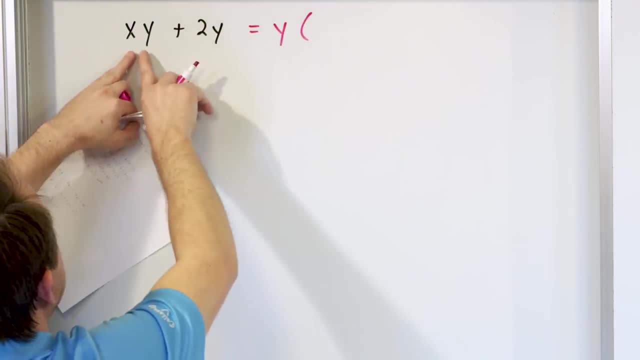 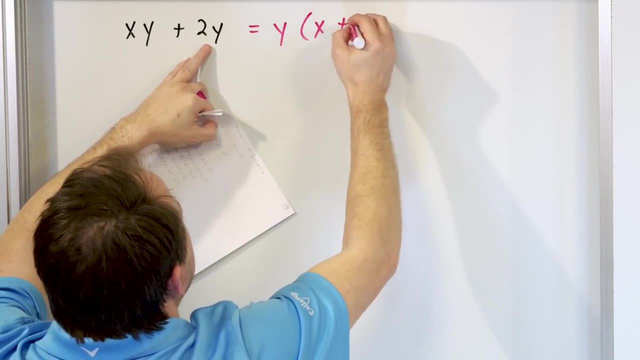 here's a y and then I just figure out what needs to go on the inside To make this term. y times something makes that term and that's x. so y times x gives me that Y times something. to give me this term means this will be a two. We've done this kind of factoring. 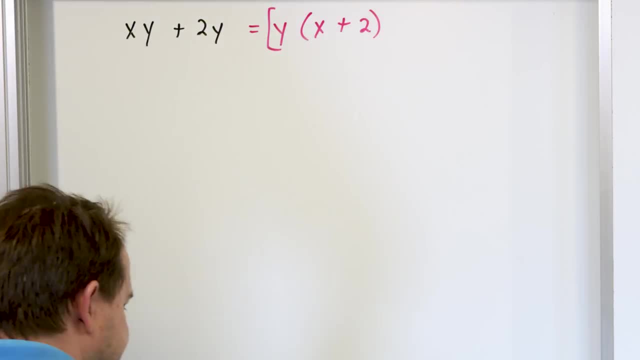 all over and over and over again there. Now I'm just doing that mostly as a review, and now I want to scoot along into what factoring by grouping really is. What if I give you the problem that's very similar to this one. We're going to change one thing: Instead of x times y plus two times y, 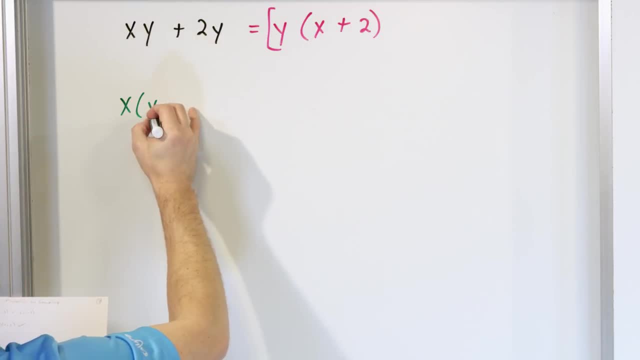 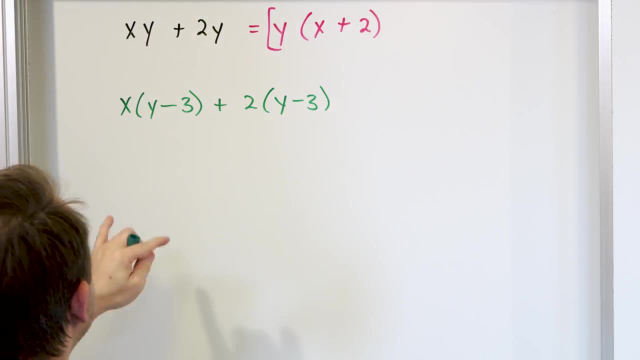 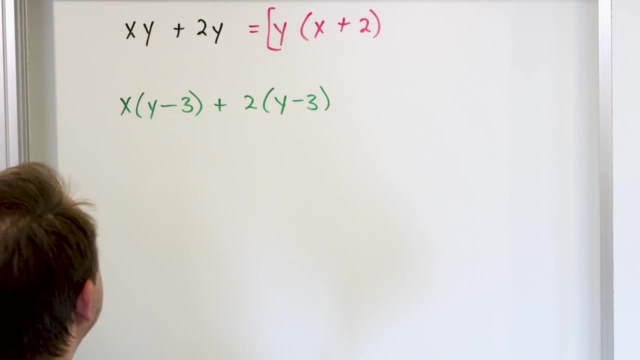 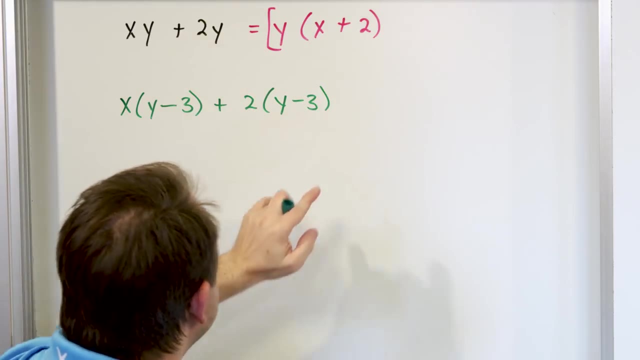 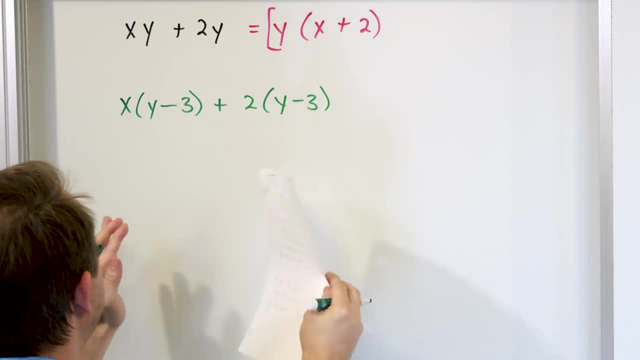 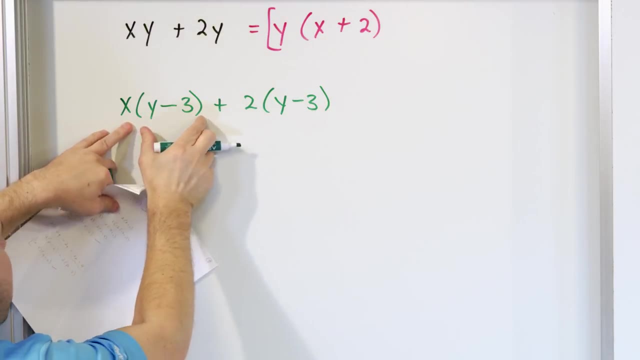 is the main idea of factoring by grouping. It doesn't look right now that there's much in common between these terms, until you zoom out and look that it's x times something and two times something. But what's common to both of them is not a single variable, It's this entire thing: Y minus three. 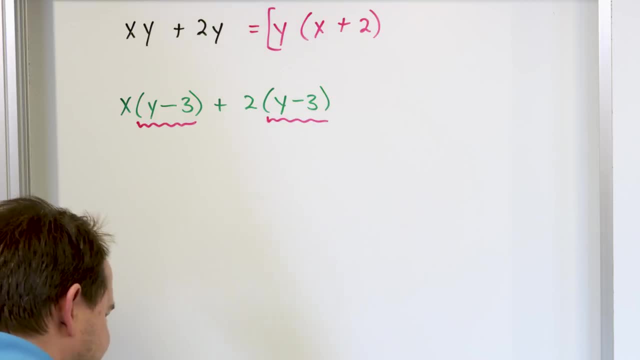 is common to both of them. So factoring by grouping oftentimes means pulling out large terms that happen to be common to both. So if you think of it just like we pulled out the y here, I can take and grab the y minus three, which is common to both terms, and pull it out. 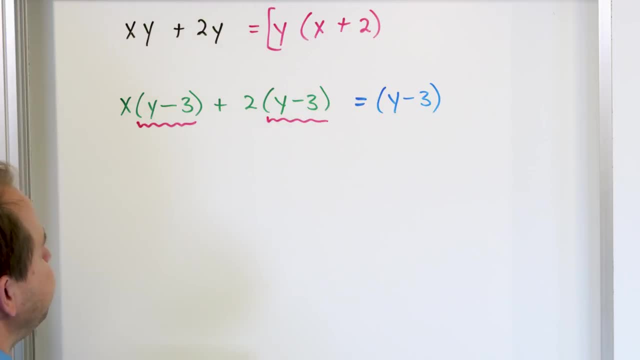 To do that, I'll wrap it in parentheses and say: y minus three gets pulled out. So then I say, all right, got to open up another parentheses. Y minus three gets pulled out. Y minus three times. something gives me this Times. what Well, it's got to be multiplied times x. 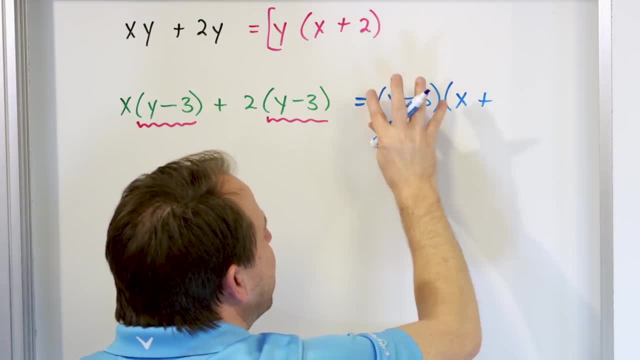 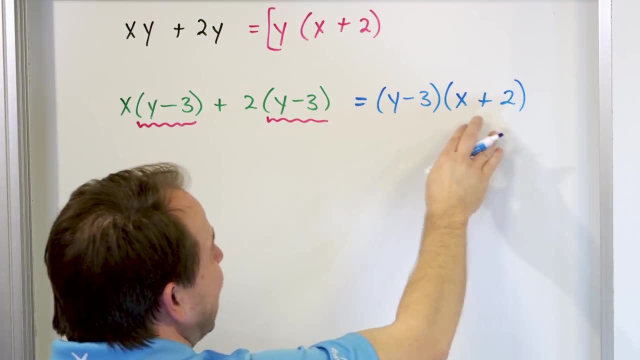 Then I have a plus sign And then y minus three has to be, as a quantity has to be multiplied by something. to give me, this term has to be multiplied by two. So you see, this looks an awful lot like a factored form, right? And this is the final answer. And if you think about it, 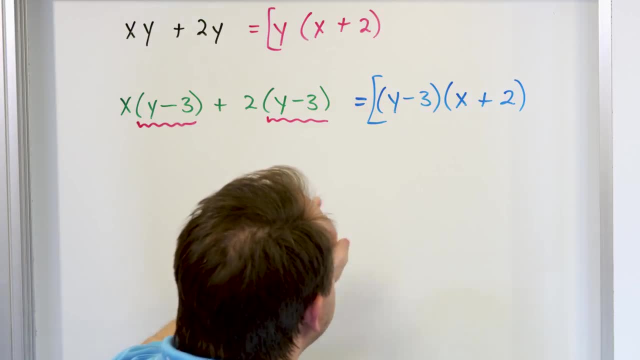 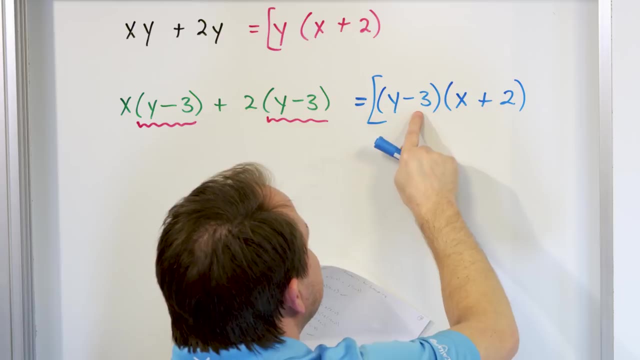 it makes perfect sense, Because what we've done in the past is I've told you to multiply these things. Here's what you do. I said: take the y times this, the y times this, the y times this times this, Then take the negative three times this, the negative three times this. I told you. 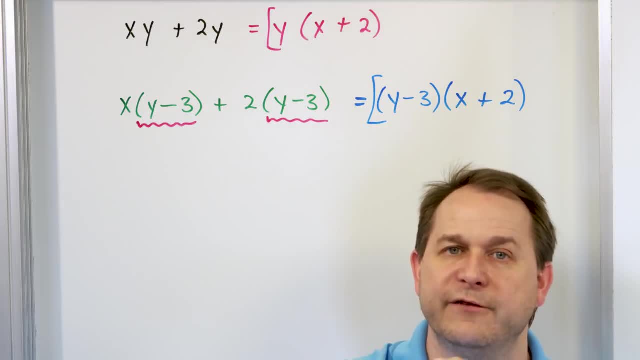 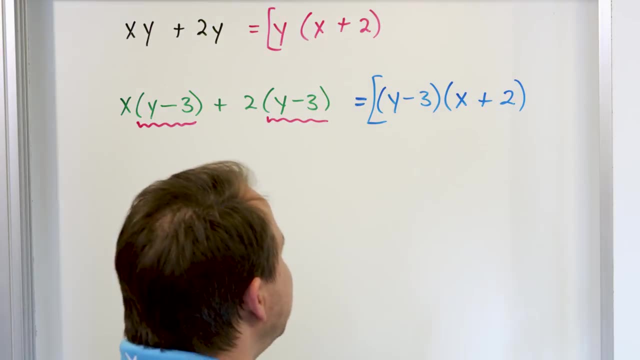 that every term on the outside needs to be multiplied individually and distributed in. That's what we talked about when we talked about what distribution really is, what FOIL is right, But you can also think about it in an alternate way. You can think of this: y minus. 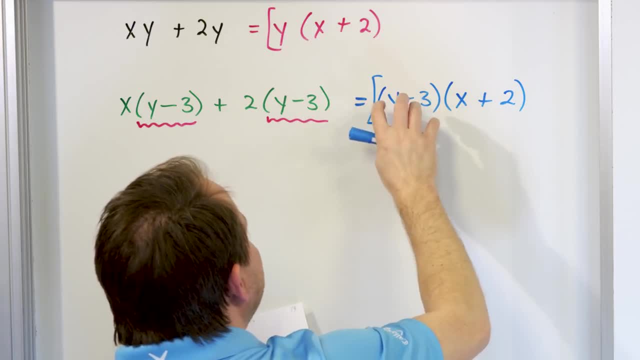 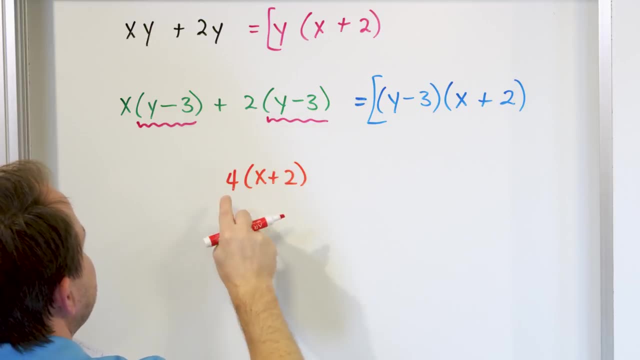 three being one big thing that's on the outside, Just like if it were just four times x plus two, the four would go in and multiply by each term. But the four is not four, It's an entire term. So it's this times the first term And also that giant thing times the second term. So that's why. 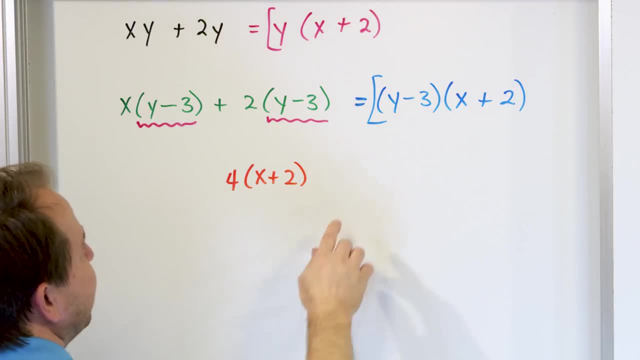 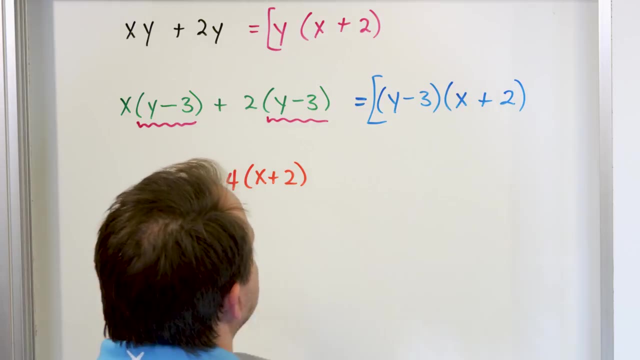 they're equivalent to one another. And if you want to blow it out even more, you could do FOIL on this and blow it all out into terms And you could distribute all this stuff and blow it all out into terms And you would see that the left and the right-hand sides are equal. So the main idea: 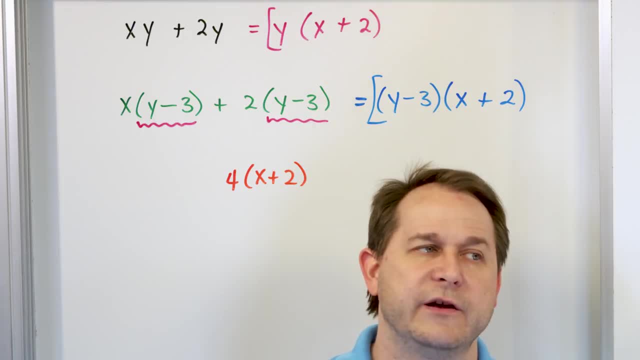 about factoring by. grouping mostly means that you would have a group of factors And you would have to look for things that are common between terms to pull out. But sometimes those things that you pull out can actually be large terms that are common to both, kind of like adjacent larger terms. 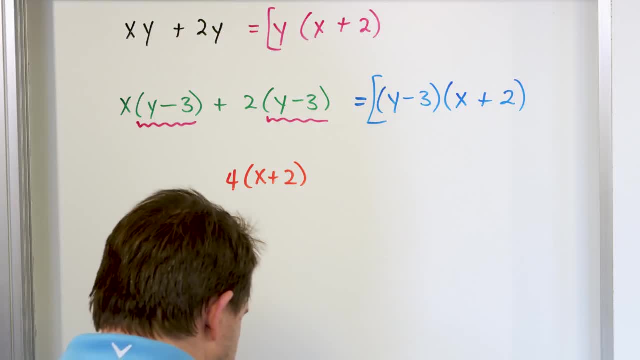 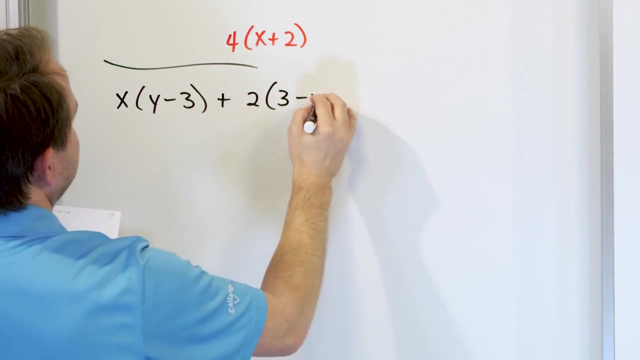 there. In this case it was y minus three. that was the guy, that was common. So let's do another one. You'll get the hang of this as we go along. What if we have x times y minus three- Again very similar so far to what we have, But then we have plus two times three minus y And we say: 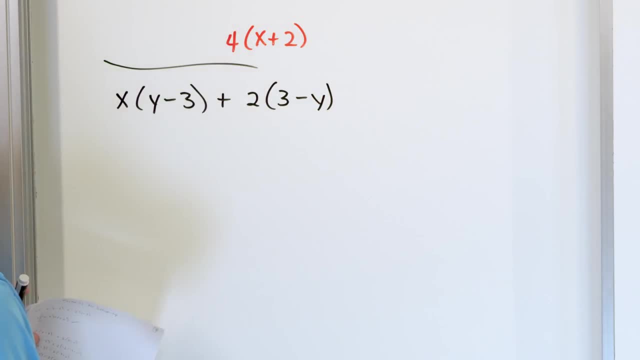 let's factor this: Well, first you think there's nothing you can do because x is here. I don't see any x's over there. I have y minus three. but I can look for a y minus three over here. I don't. 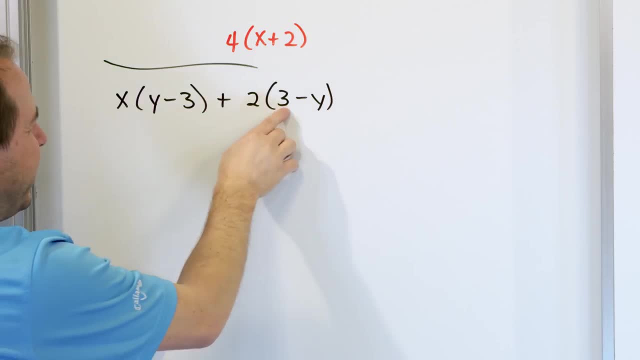 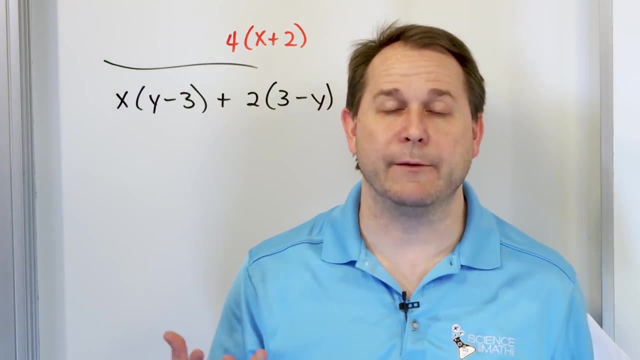 see that, And there's no two common either. I do see that there's a three here And I do see that there's a y here, But it doesn't look like it's in a form that allows me to pull it out Now. 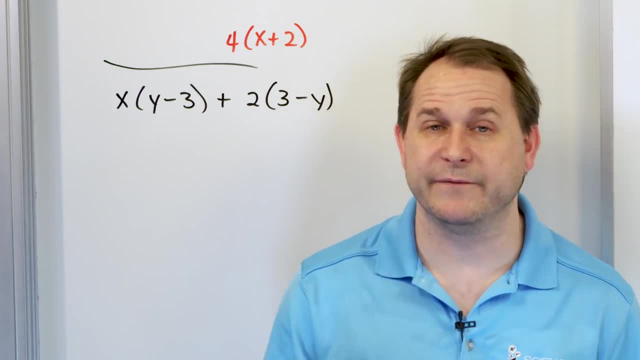 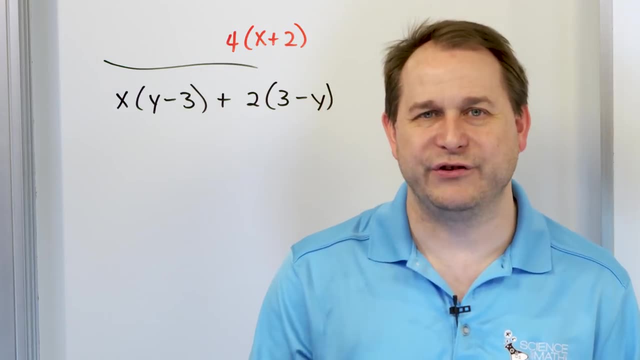 here's the secret of algebra and the secret of all math and physics and chemistry that you're going to learn beyond now. What you've learned is that you're going to be able to pull out up to now is the rules. You've learned what is legal to do right Now, as you go farther and 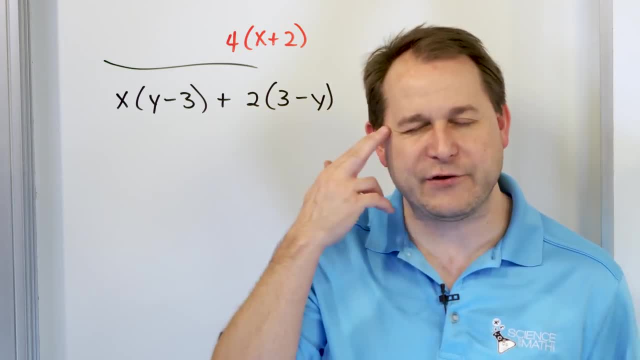 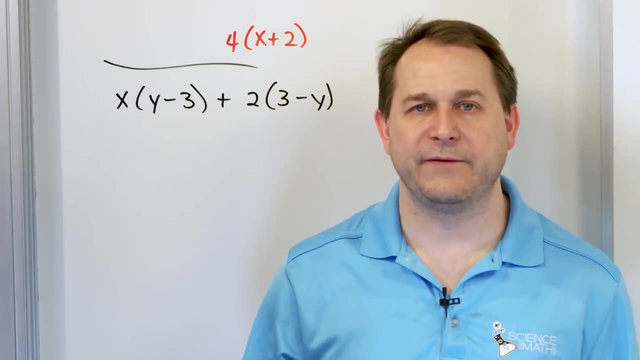 farther into learning math. what you need to do is use the rules that you have in your brain to do whatever you can to make the thing into the form that allows you to simplify further. In other words, your problems from here on out are probably not going to tell you exactly how to simplify a. 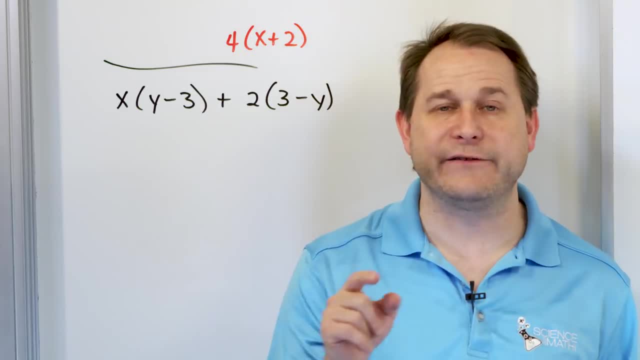 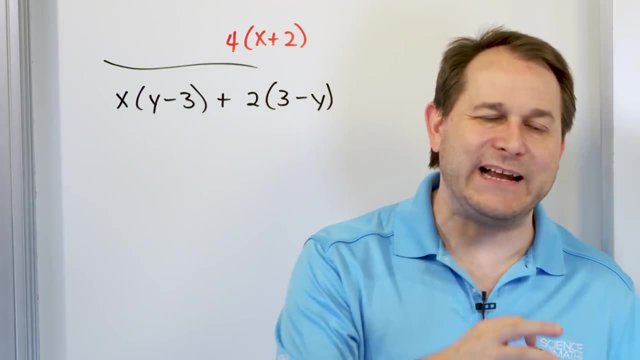 term. But what you know that you can do is you can manipulate any term there using the rules of algebra that are known to you right To transform it and write it in a way that lets you then do what you want, In other words, 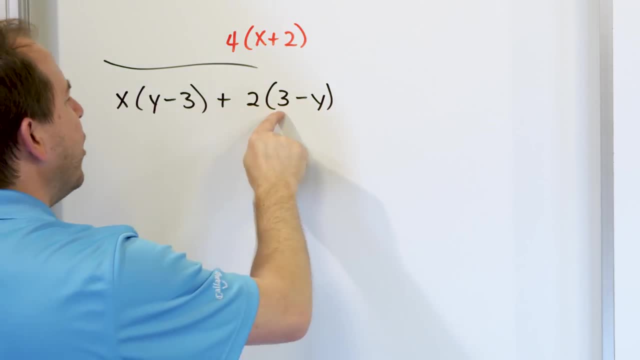 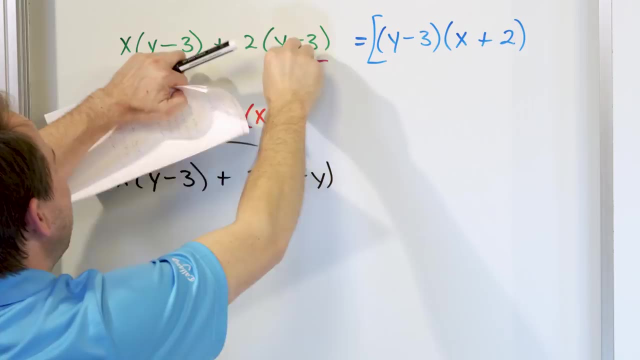 it sure would be nice if this was y minus three and this was also y minus three, Because if it were y minus three it would be exactly the same as this problem, And then I could pull this giant term out like I did before. But oh, unfortunately it's not like that. It's three minus y, So what? 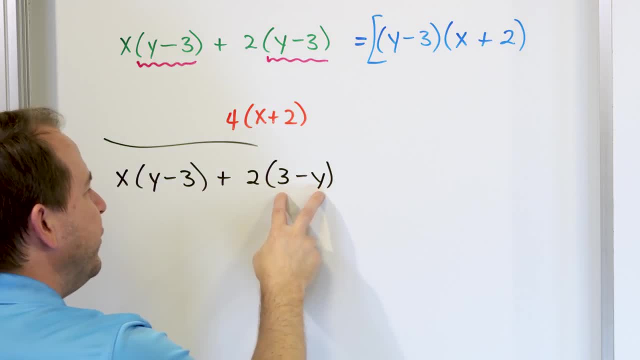 do you? do You realize that you can change this using the rules of algebra to make it into a y minus three? Then you can then factor it out. So what do you? do You realize that you can change this using the rules of algebra to make it into a y minus three? Then you can then factor it out How. 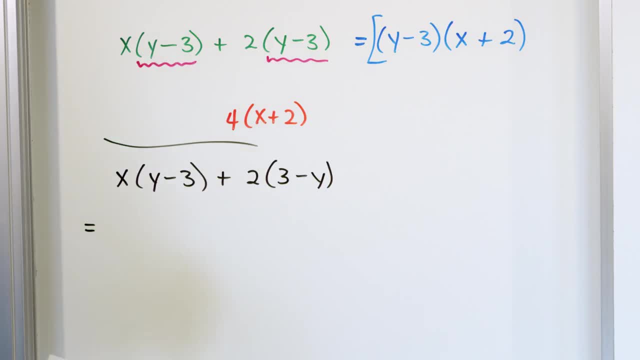 do you do that? Well, you go step by step. The first one we're going to leave alone. We're not going to touch him at all because he's already in the form we want. But what would happen is what would happen if we attempted to pull out inside of here. Let's write it as you know. let's just. 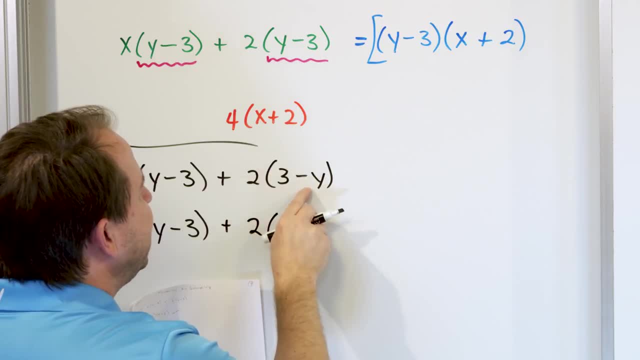 write it with parentheses, I guess. What if we pull out a negative one from each of these terms here? Just forget about the rest of the problem, Just focus on this. What if we pull out a negative one from here? Then we'd have a negative one, but we'd have a negative one from here. So what if we 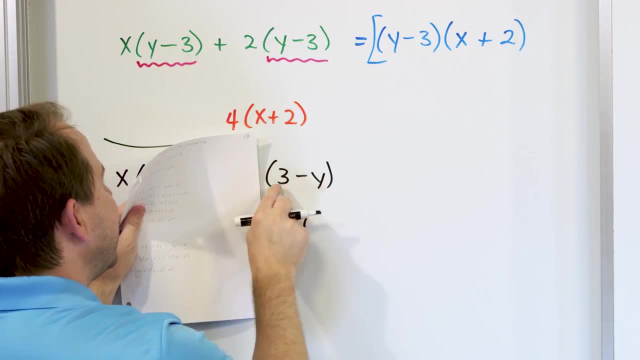 pull out a negative one from here, Then we'd have a negative one from here, Then we'd have a negative one, but we'd have to open up a parentheses. And if we did pull out a negative one, then on the inside, 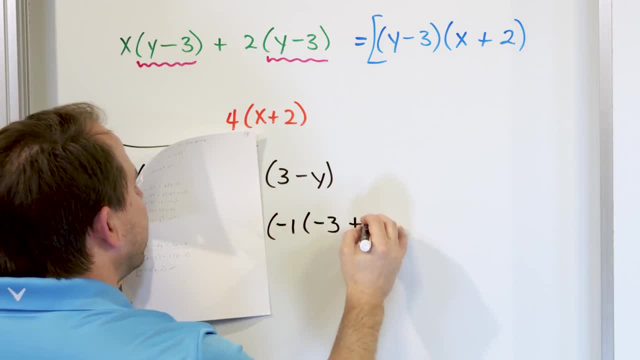 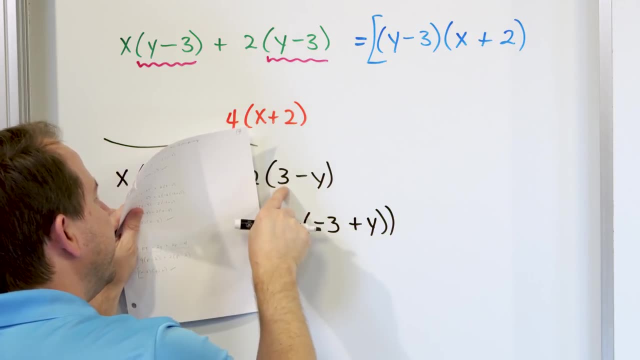 we'd have a negative three And then this would turn into a positive y. And before your mind explodes, think about what you're doing. All you've said is that this times this has to give me this positive three, And it does Negative times. negative gives me positive, Negative times. 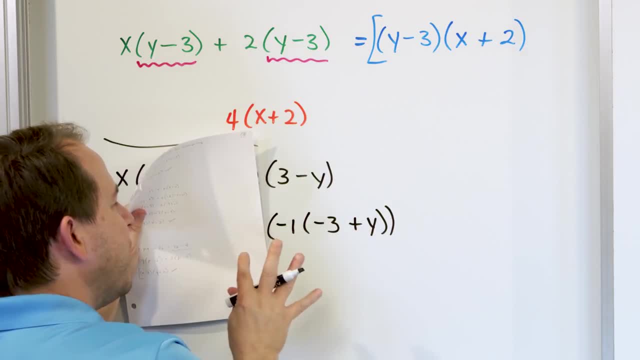 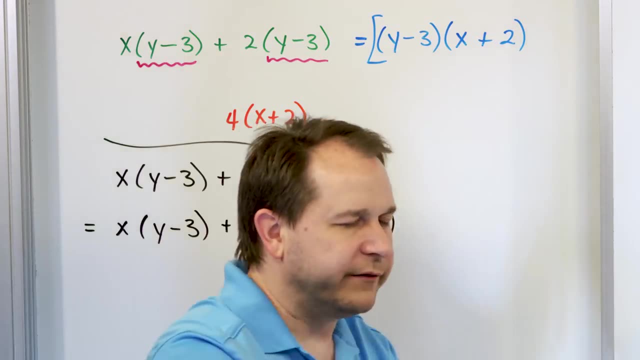 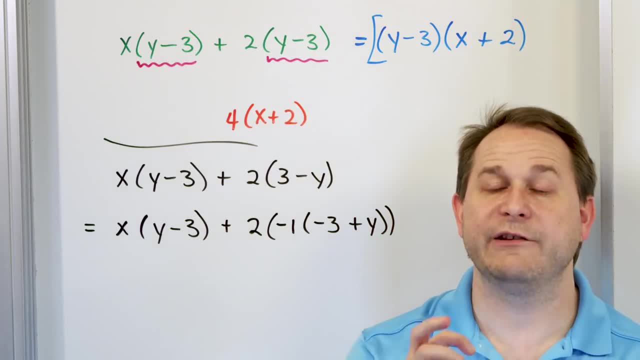 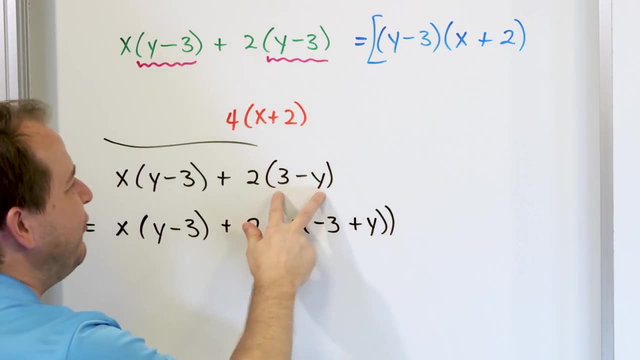 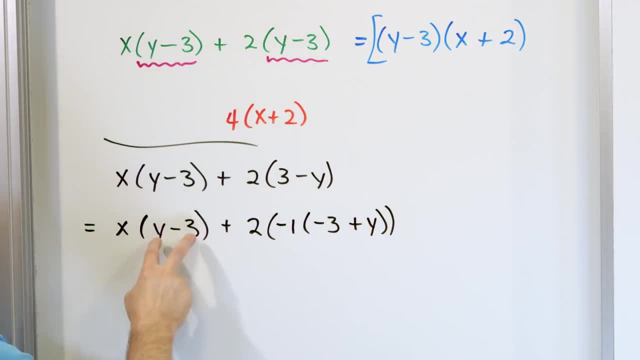 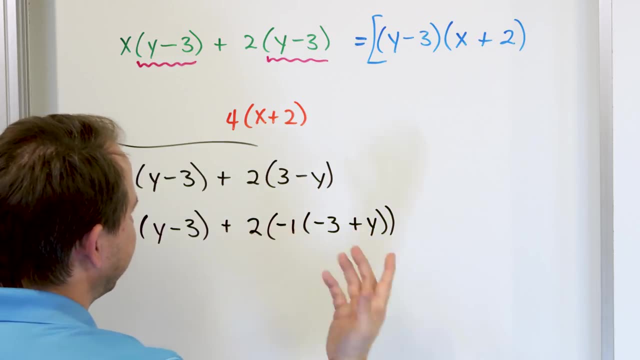 change the sign of everything on the inside. in the next step you're going to see, I'm going to be able to write this as y minus three, which is going to match what I have Now. in order to do that, I had to factor out a negative one, which was some work. Let's get through the problem. 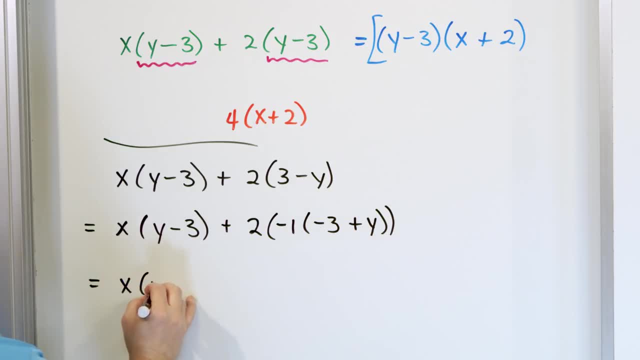 and then we'll finish the rest of it and we'll summarize. What we have is x times y minus three. This negative one's factored out, but it's multiplied by the two. So what you end up having is minus here two times. 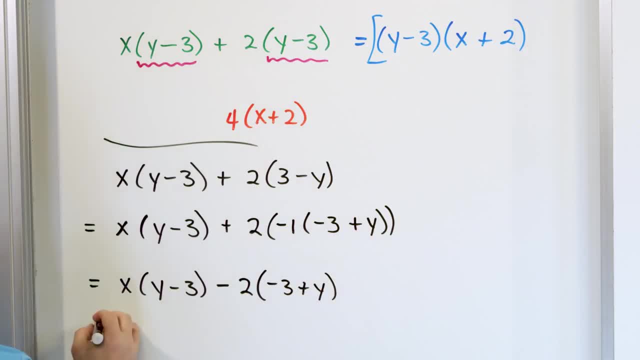 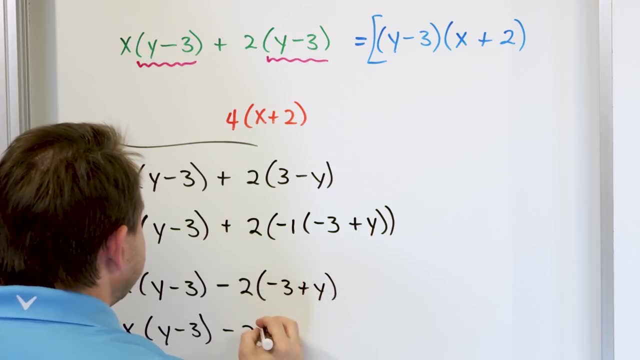 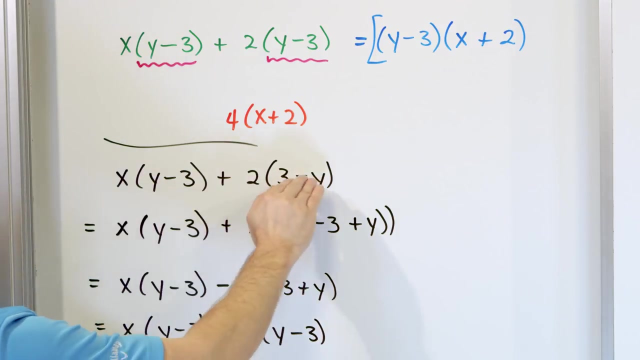 inside here, negative three plus y, And then in the next step, what you can do is, since it's negative three plus y, I can change the order of the addition. That can happen any time I want, but it'll be y minus three. So you see what I have now. It's not exactly the same as what I've written in. 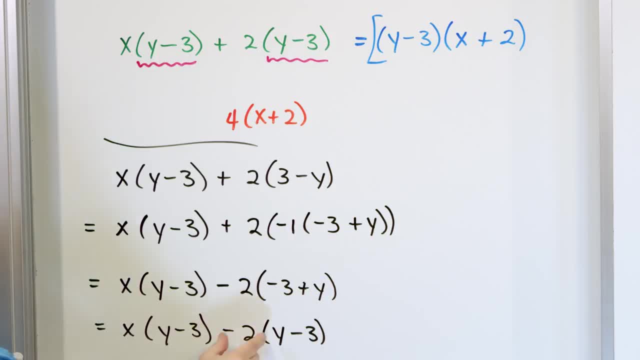 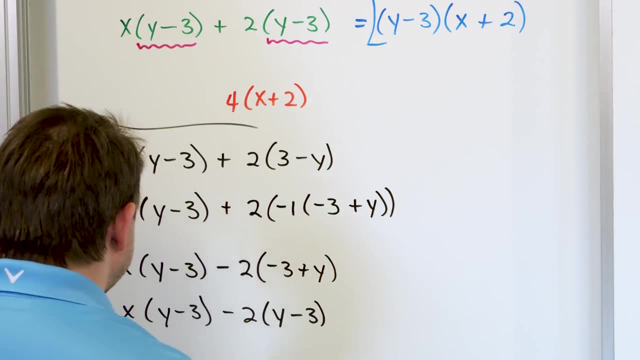 the beginning. but now I do have a common term- y minus three, and another common term, y minus three. Those two terms can be pulled out as a common factor, just like I've been doing for all the other problems. So if I do that- and I'm going to pull out as a common factor y minus three- 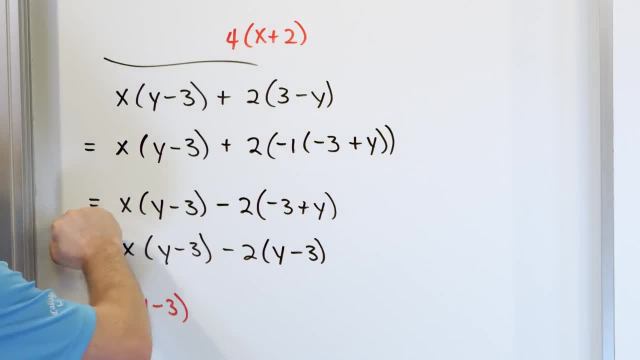 then you have to pretend for a second. okay, what if this were just something I pulled out? This times, something is going to give me x, but this is what I'm trying to reach, so I'm just going to have to put an x here, right? And then there's a minus sign here, so that's going to go. 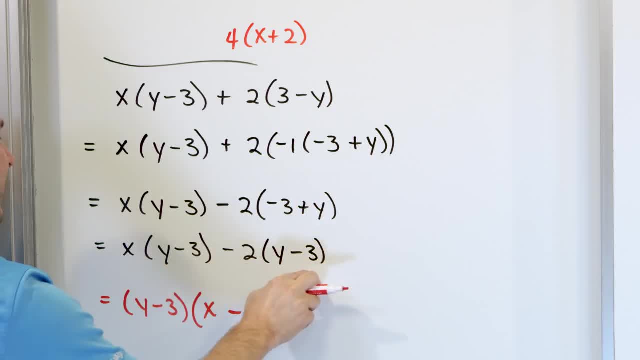 here, This times negative, something is going to give me this: The only thing that works is a two. So you've got to think of it differently than FOIL. you've got to think of it as this giant term times. the x gives me this- This giant term times. 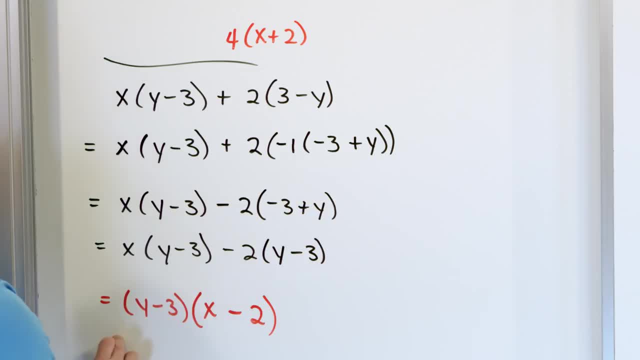 negative two gives me this. So this is therefore exactly equivalent to the line above it, and you trace your steps back, which means everything is equivalent to this. Now, to totally prove it to yourself, you can multiply all this out. and then you can multiply all this out and you would find. 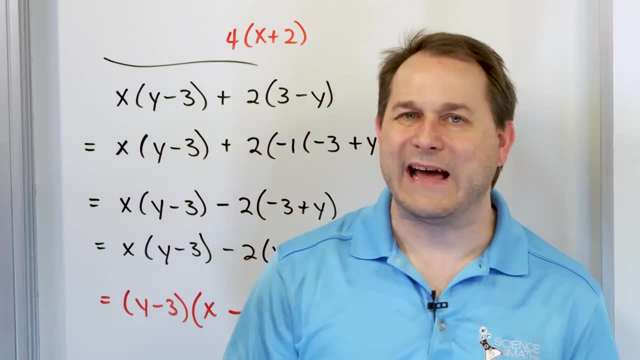 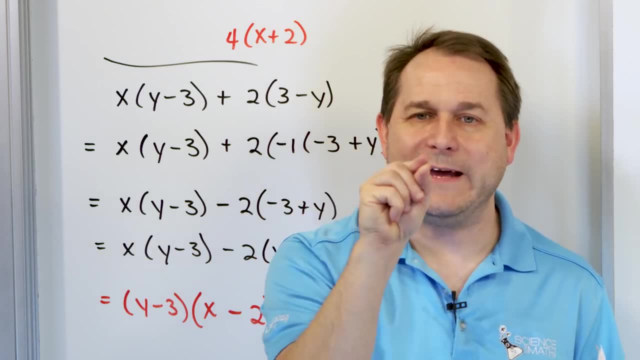 that everything's the same. But the trick to math, to trig, to calculus, to physics, to chemistry, to anything, is to make sure that, between every single step, what you are doing is is that you are doing everything that you can to make sure that everything is legal. Then you build. 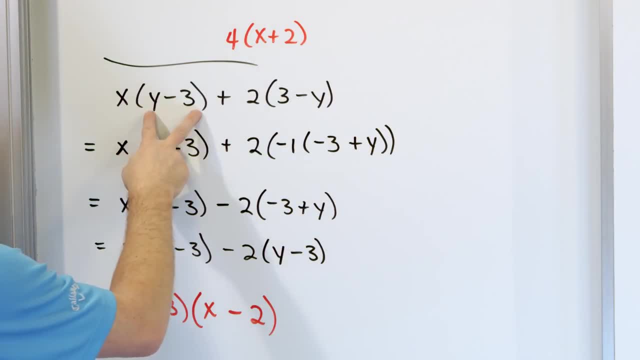 a chain all the way to. the answer that you know is then bulletproof right. So we start at the top. we say, well, this is y minus three, this is three minus y. They're pretty close, but they're not. 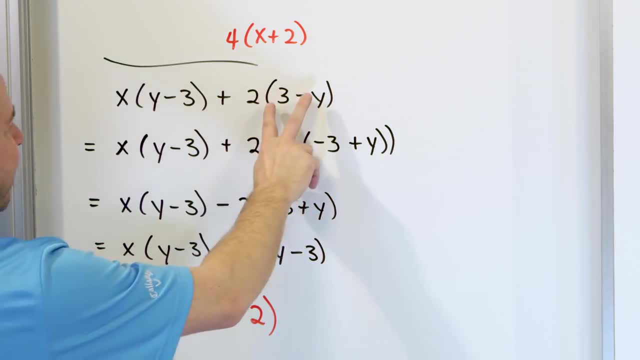 quite there. So I want to change this to make it y minus three. How can I do that? I can't just do it. I can't just change the problem. But what I can do is I can factor out a negative one, That is: 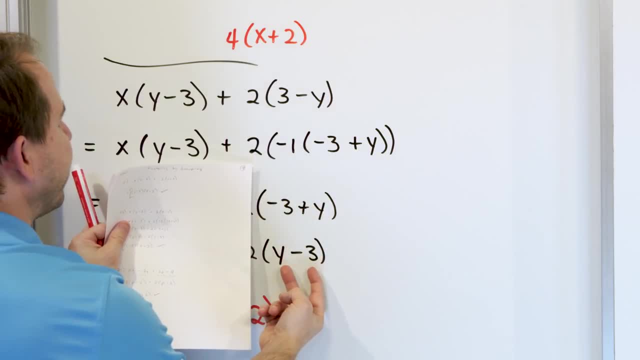 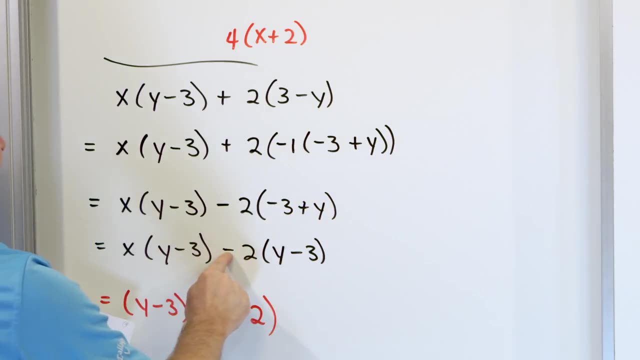 going to change the sign of everything inside, which, in the next step, will allow me to then flip it around to y minus three. So that's going to be multiplied out here, So this becomes actually negative two. So this has a minus sign, whereas the original problem had a plus sign. right So? but these are exactly equivalent. 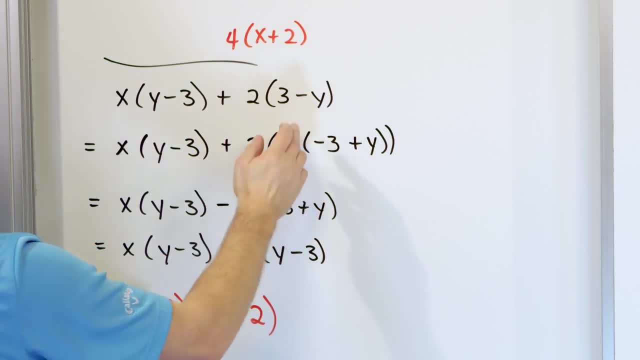 to one another, because even though this is now negative, I changed the sign of what was on the inside, So everything is equivalent. Then I take the y minus three, I pull it out: x minus two is what's left over, And that is what factoring by grouping is. It's looking for larger terms than 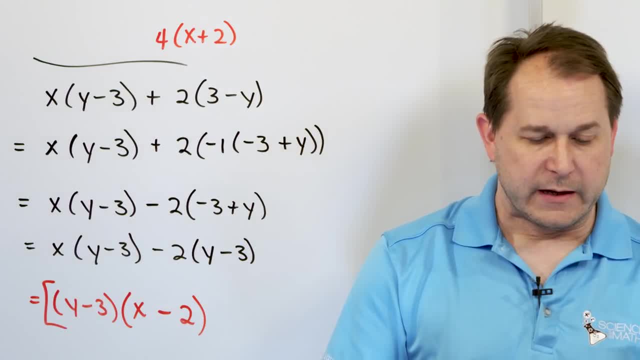 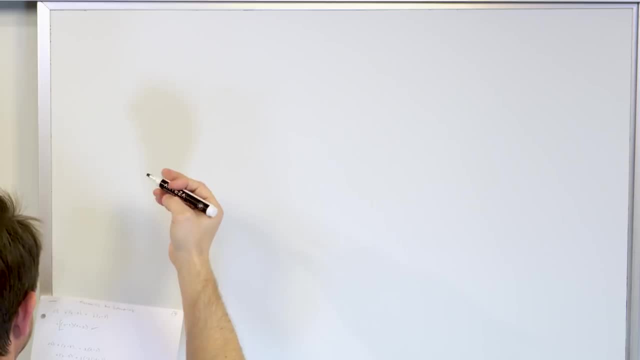 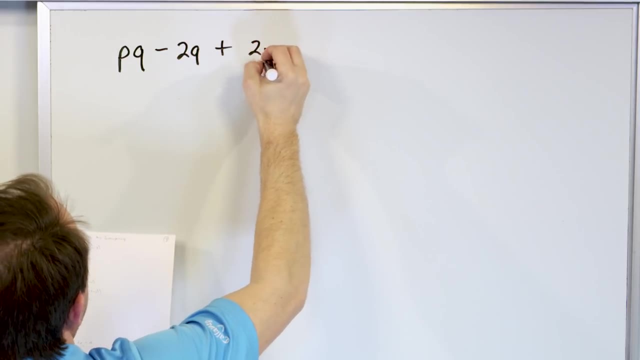 the ones that we've done in the past in order to pull out larger terms and simplify them All. right. now let's take a look at another one. This one's actually a little easier than that: one P times q minus two times q plus two times p minus four, And I tell you, factor that. Well, the first. 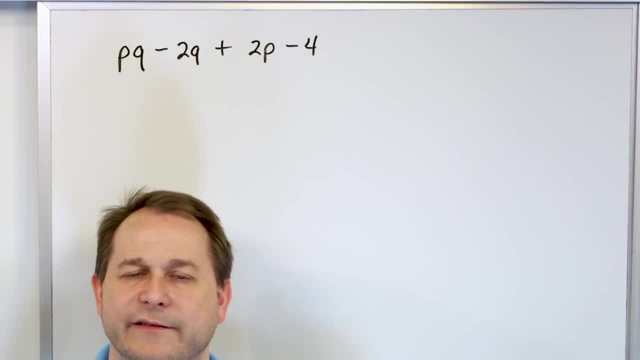 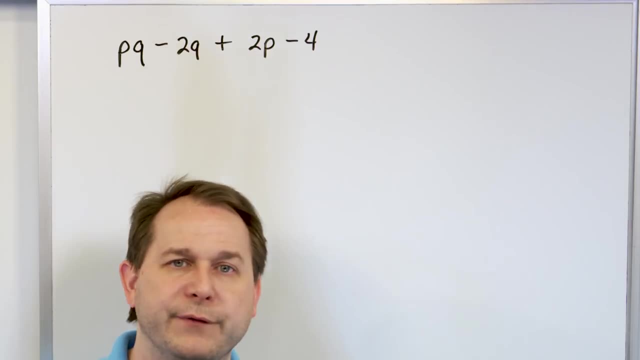 thing you do. I know you're in a factoring by grouping lesson so you want to try to look for factors that are, you know, large factors or whatever. But the very first thing you do, if I tell you just factor something- is you try to look for things that are common to all the terms. So 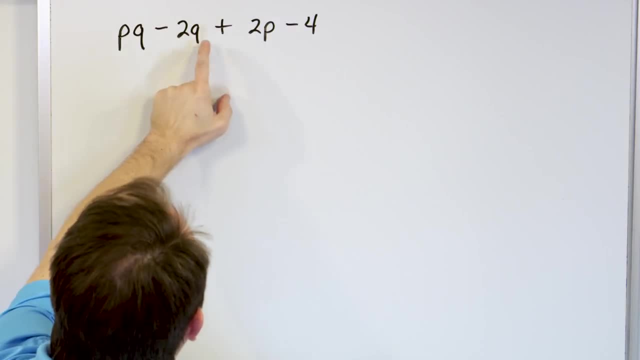 then you say, all right, here's a p, here's p, there's no p here and there's no p there. so I can't do that. And you say, here's a q, here's a q, no q's here. can't do that. So you're kind of. 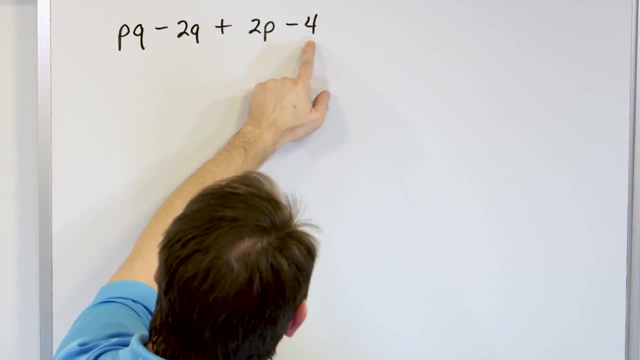 discouraged. Then you say: well, there's a two, there's a two, I could factor a two here, but there's no two here, so I can't do that. And you look at four, and you can't do that. So you think 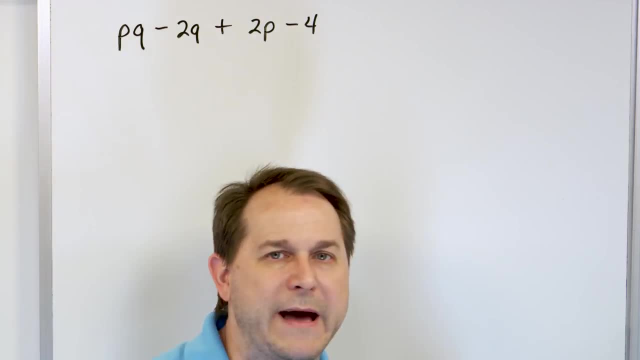 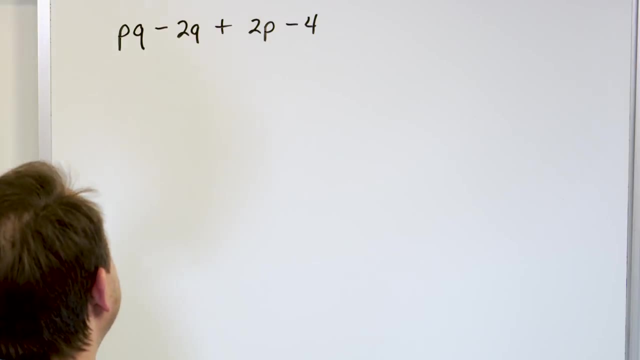 you're stuck. But then you realize sometimes math is about zooming into smaller parts of the problem and trying to factor smaller little things just to simplify it a little bit. So instead of trying to factor the entire problem, you're going to try to factor the entire problem. So instead of trying to 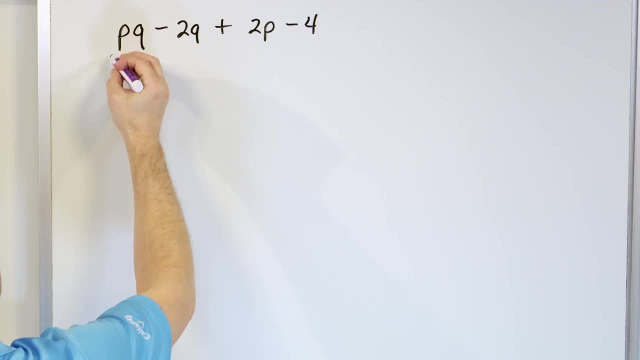 factor the entire expression. I only want you right now to focus on the first two terms. Forget about this stuff. Factor these first. Well, there's a q here and a q here, So I could pull a q out of just those two terms And this times something here would be p to multiply to give me pq, And 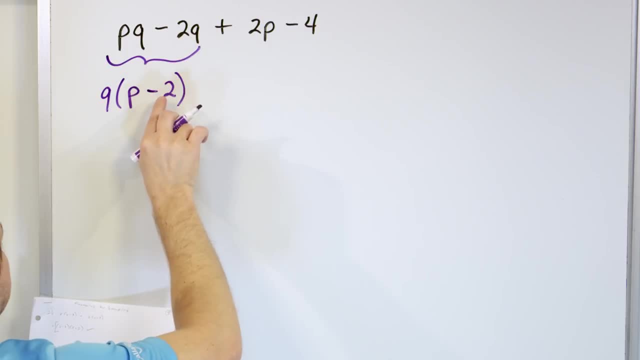 then here would be minus two, because I'm trying to get negative two q there, negative two times q. So you multiply this into both places, you recover those first two terms. Now what you have over here is still exactly the same. So you can't do that, You can't do that, You can't do that. 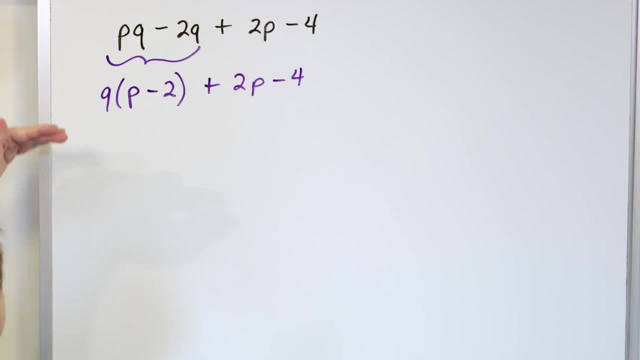 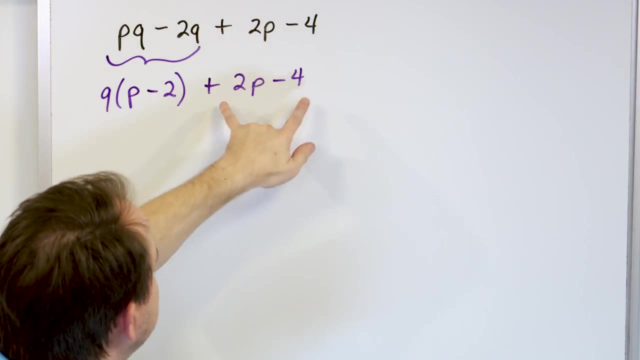 That doesn't go away. I hope you agree that going from this line to this line are equal to one another. All I've done is factor out a term from the first two right, And then these just come along for the ride. They're still added. They just haven't done anything with them, But I factored. 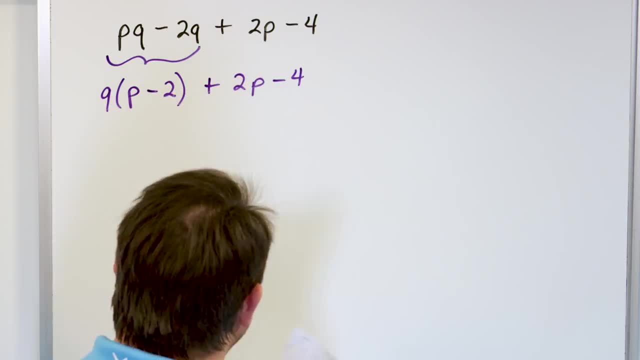 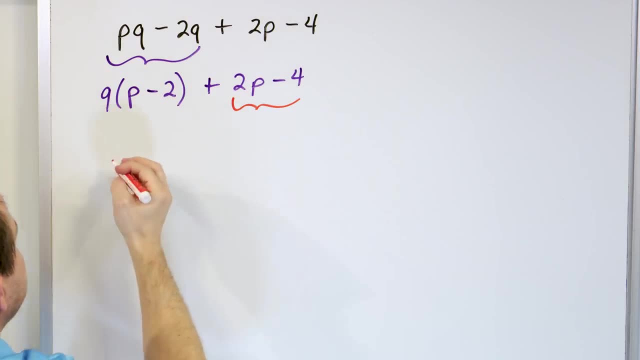 out a q from the first two terms And then I look at the second two terms and I say, wait a minute, I can just focus on those. And I see a common factor here. I could pull out a two from here and from here. So let me rewrite the problem: q times p minus two. that stays the same, But I'm 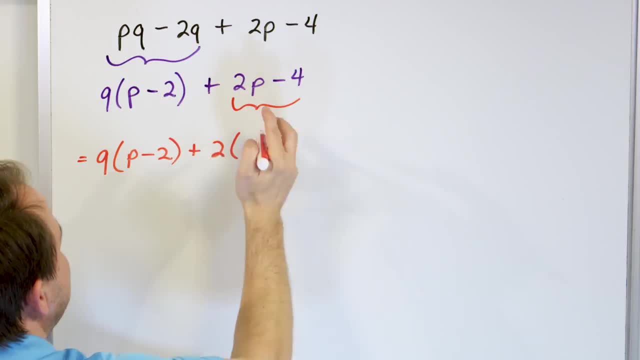 going to factor out a two from here and from here. So let me rewrite the problem: q times p minus two from here, And if I do that I need to have a p on the inside here and a minus two on the inside. 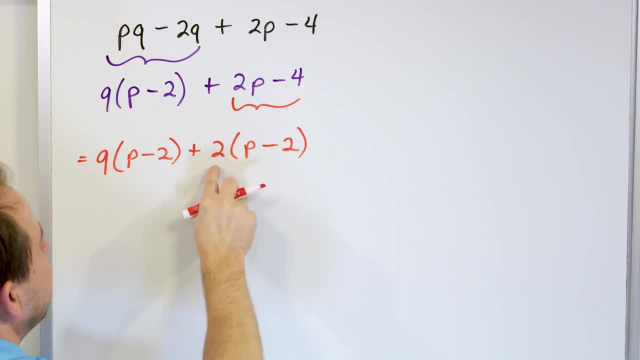 there Two times p is this? Two times negative two is this? So this is the factored form. And then you're about to circle your answer and you're saying, well, I did pretty well. But then you realize, wait a minute, there's a quantity p minus two here and the exact same quantity p minus two. 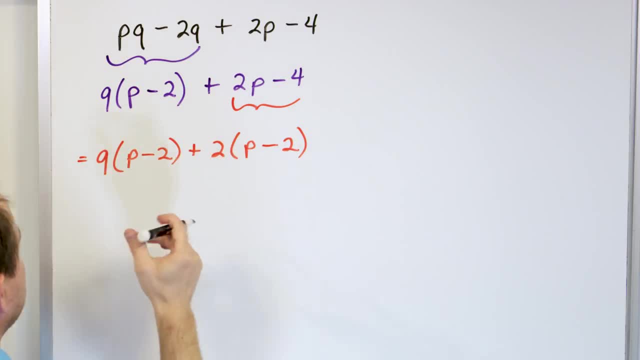 here. So actually I can pull out this entire large term called p minus two. But then I have to figure out what goes in here to give me multiplied. Well, just a single q, multiplied by that would give me that And then plus sign because of this. 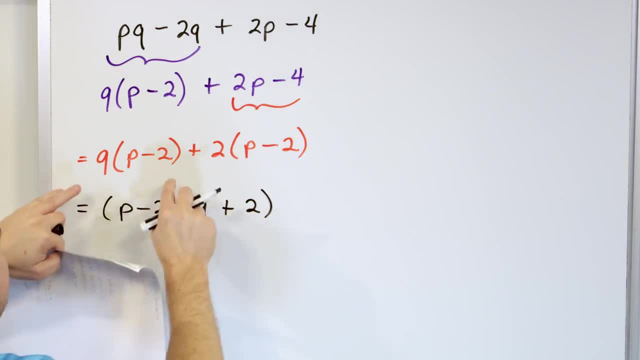 two here. So then, this times this quantity would give me this. This large thing times this quantity would give me this. This is the final factored form. I don't care who you are, unless you are a genius, super, algebra, crazy, awesome person, You are never, ever, ever going to be able to. 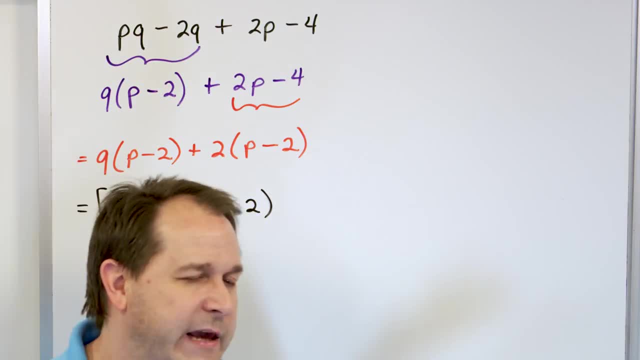 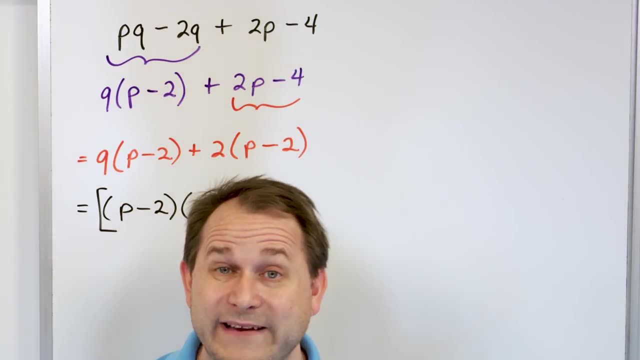 look at this problem and understand like that that it's going to factor into this. I can't do it. I don't know anybody that can do it, unless you're just really really good at seeing patterns, And that's fine. Maybe you are, That's great. For the rest of us, you have to take it step by step. 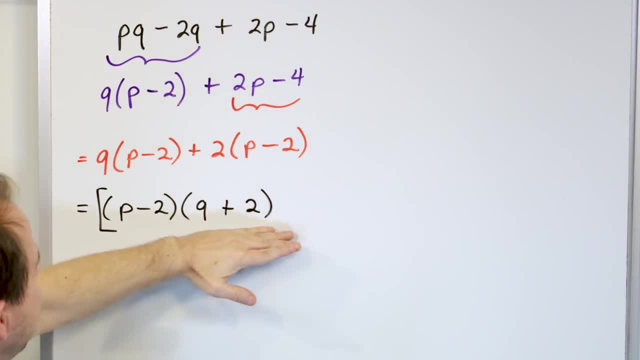 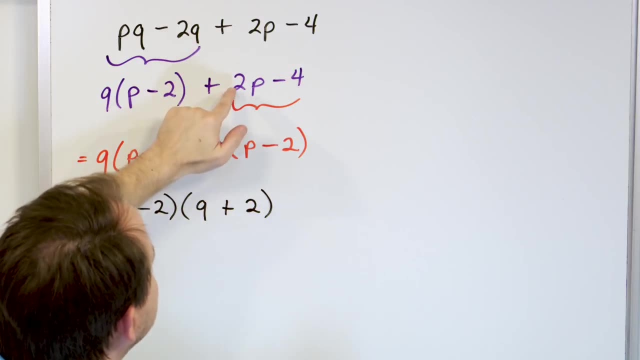 When I do this step of the problem. I have no idea that it's going to come out to this, But I do know that I can factor out the q from the both from the first thing here. Then I looked at the last two terms and said I can factor out a two Right around. here is when I realized: wait, a. 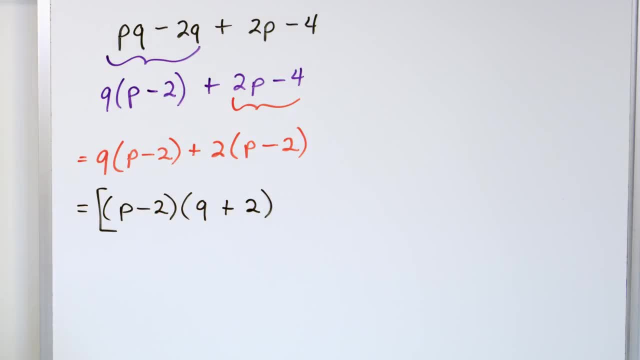 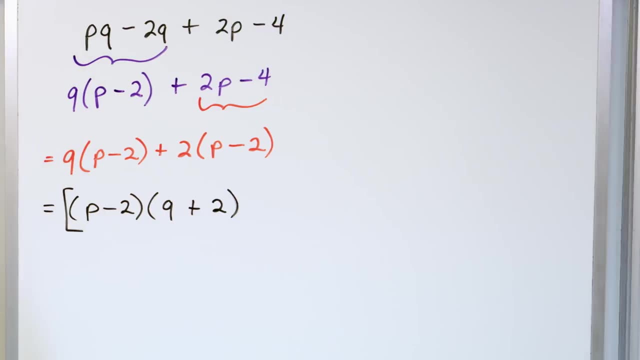 minute these are going to actually match. Then I can use factoring by grouping to do the final part of the answer: p minus two, q plus two. Final answer: All right. One more problem. This one's a little challenging but it's not that bad. 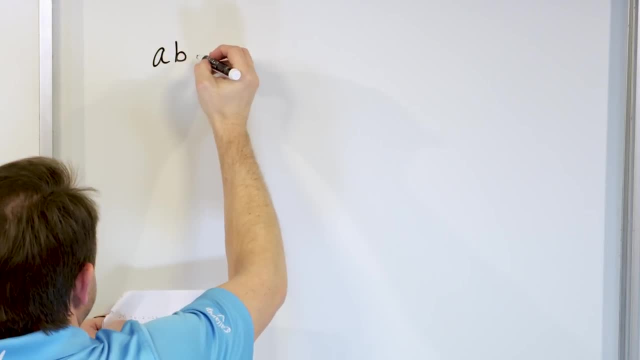 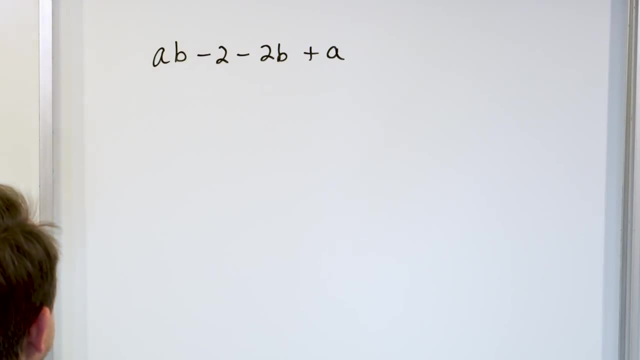 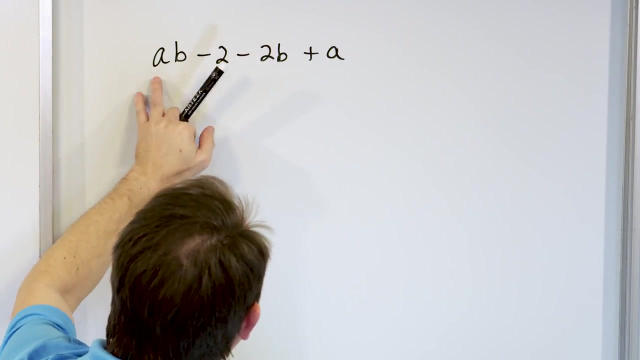 really We have four terms. We have a times b minus two, We have minus two b plus a. And I just tell you something: general Factor this expression. First thing you do is you look for commonality among everything. I have an a b. There's no a b here, So I can't pull out an a b immediately. 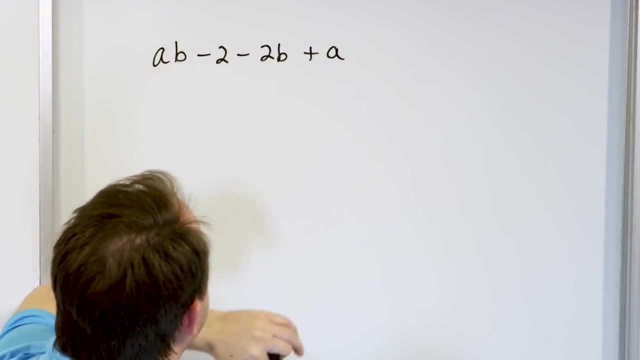 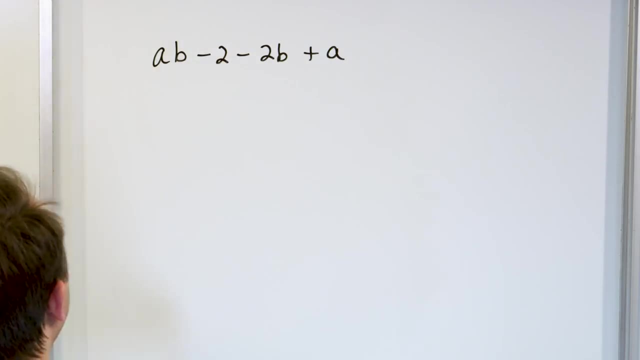 from all terms, because I don't even have a b here and I don't even have an a here. I don't have an a here either. Same thing with the numbers. There's nothing common here. So then you start doing the same sort of thing. You start saying: what can I pull out from different? 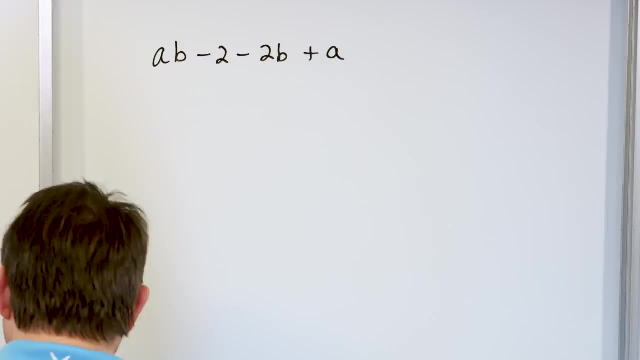 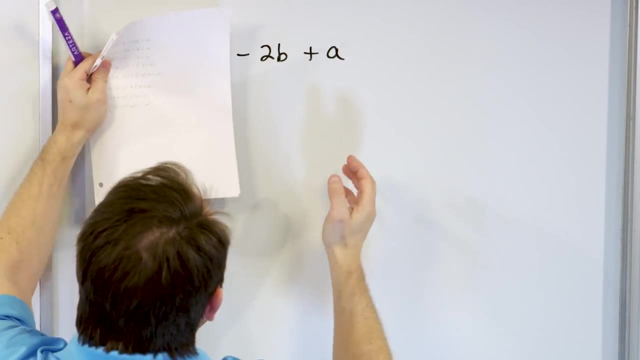 places Right. And in this case I'm looking at these first two terms like we did before. We kind of zoom in on the first two terms, but there's nothing common here. Then you look at these last two terms and you realize there's nothing in common there, And then you start to really get. 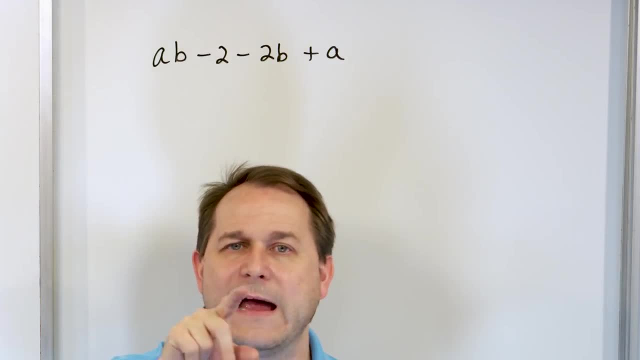 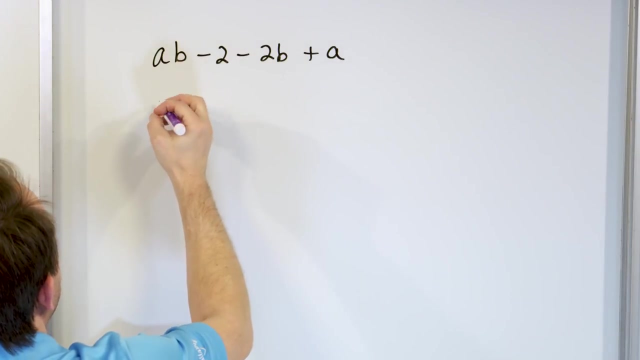 panicked because you don't see anything. But then you realize when things are added or subtracted, you can actually rearrange the order of a, two. So I'm going to do that. I'm going to do that. I'm going to say: well, what if I just change it to a, b and then this two b, I'll just move it next. 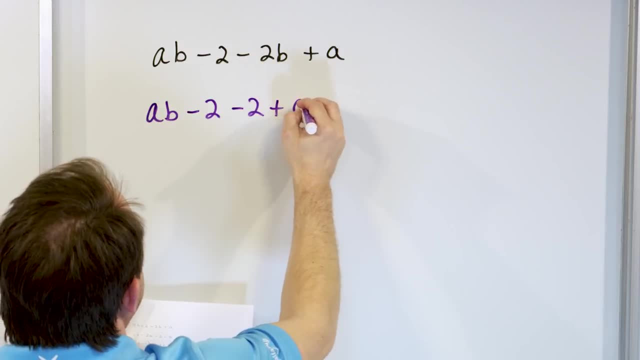 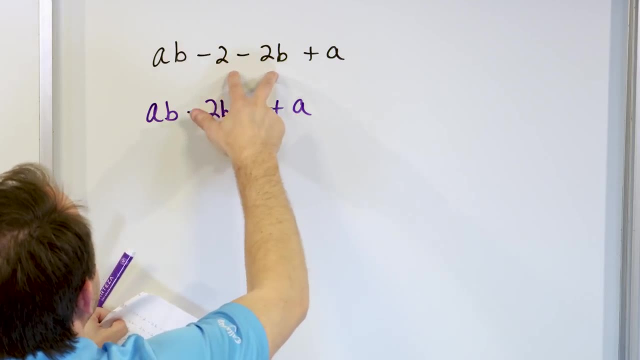 door. I still have the minus two and I still have the plus a. All I've done is take this and move it. Oops, I forgot something critical. B. I just take this and move it next to the a. b, The minus. 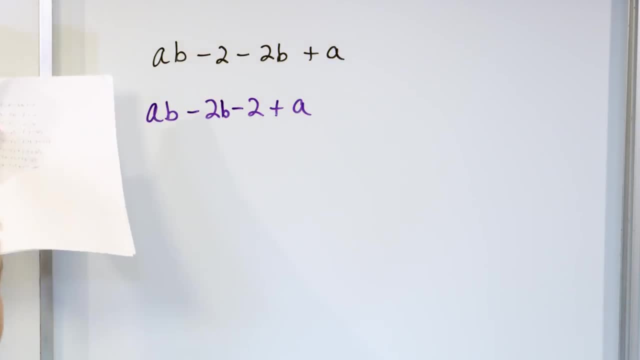 two just gets moved close to the a, but they're all going to it's equivalent to a- b. So I'm going to move this to the a- b And then I'll say, well, let's focus only again on the first. 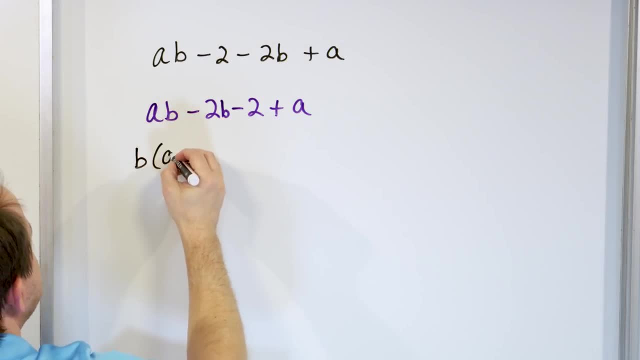 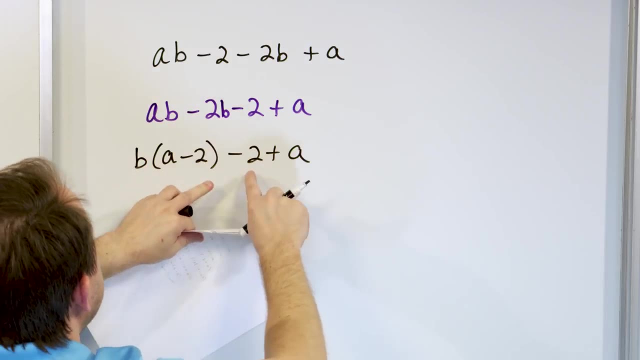 two terms. I have a common b, So I can take that out. A minus two is what I'm going to get. How do I know that? Because b times a gives me this, B times negative two gives me this. These terms have been written down directly. I haven't even done anything with them at all. 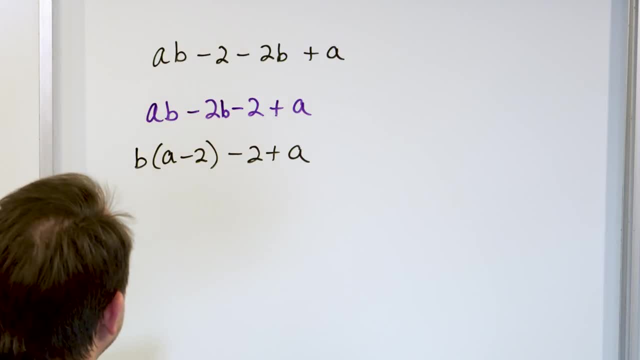 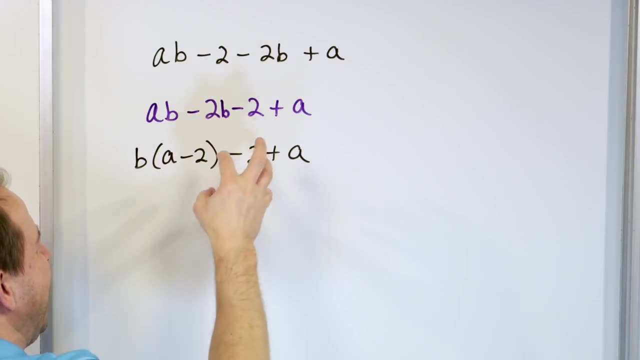 So then I say, gee, this looks pretty good, but I think I'm done. I don't really know what else I can do. This is a minus two and this is negative two Plus a. This looks kind of similar, but it's not the same. I can't grab these terms and pull. 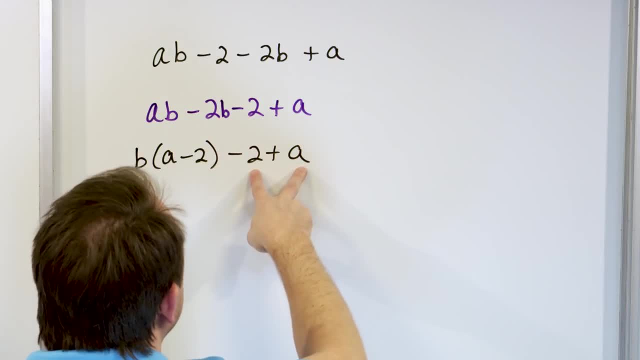 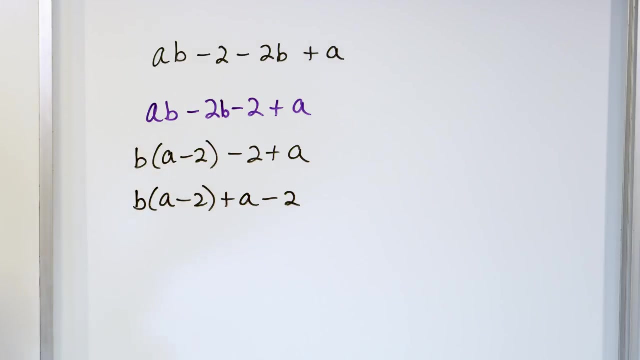 them out, because a minus two would need to match a minus two exactly over there. But then you realize: well, wait a minute here. Negative two plus a is exactly the same thing as plus a minus two, right? When you think about it, when I flip this around, 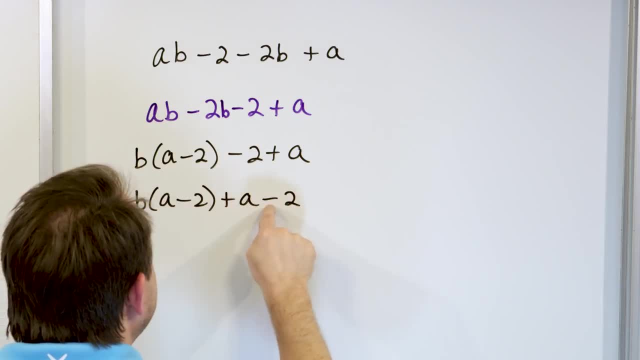 it's just subtracting two, adding a, which is the same as adding a and subtracting a. So I'm going to take this and move it next to the a- b And then I'm going to subtracting two. So to make it a little more clear, I can write it like this: b, a minus two. 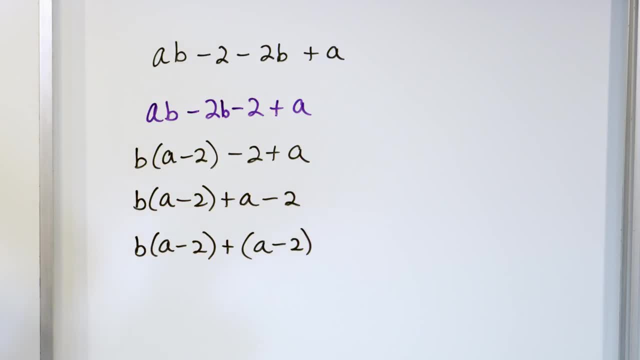 plus, I can just put parentheses- a minus two, That's fine, just to help you visualize the grouping. So now you can see it a little more clearly, right? This is a common term. This is a common term. So then I'm going to factor out the common term, which is just simply a minus two. 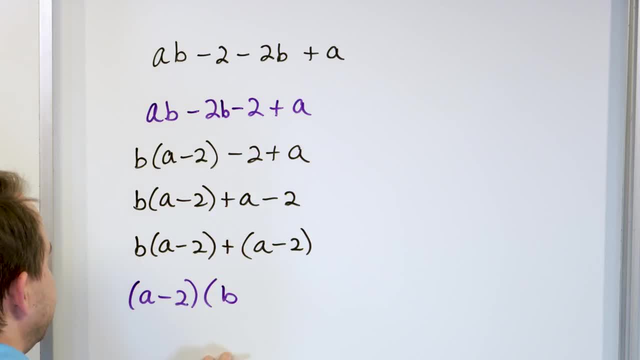 Then it would need to be multiplied by something to give me this, which is just going to be bb, And then it would need to be multiplied by something to give me the same thing here, which means it needs to be a minus two. So it's a minus two times b plus one. And if you absolutely want to just check yourself and make, 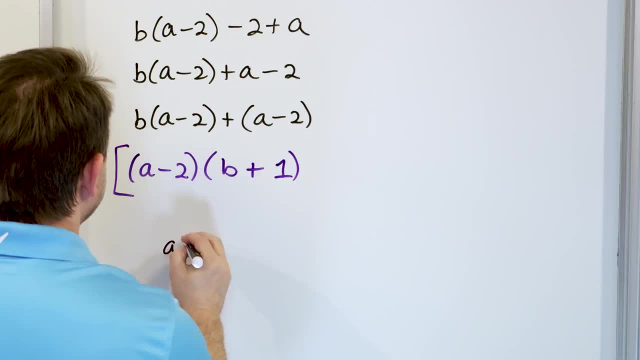 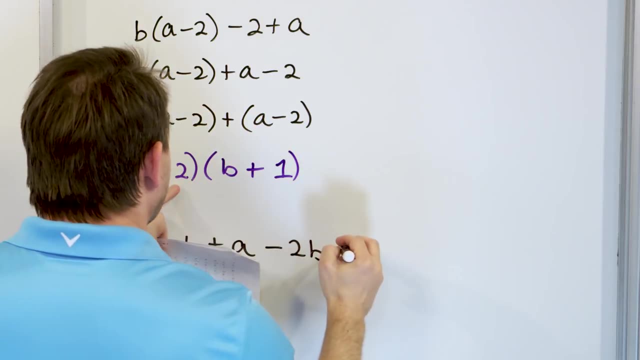 sure it's right. that's no problem. You can do that. a times b is ab. a times one is a Negative. two times b is negative. two b Negative. two times one is negative two ab. the minus two is at the. 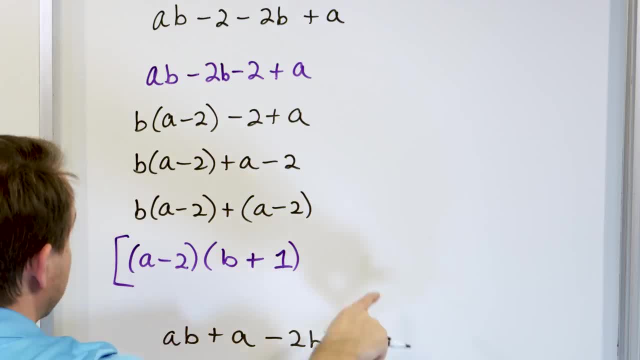 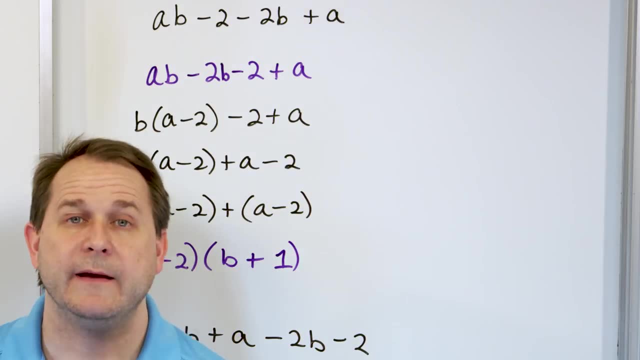 end here. The negative two b is here And the plus a is here, So they're out of order, but they're exactly the same as what we started with. So this is the factored form. All right, That's factoring by grouping. Basically, you might have to rearrange terms. 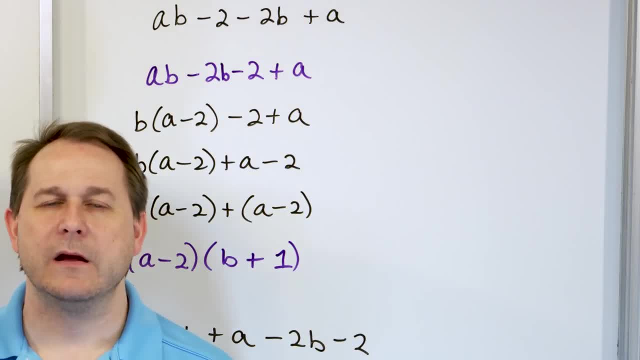 You might have to manipulate things, factor things out a little bit, But ultimately you're looking for larger subsets of things that you can then pull out right, That you can then pull out. We have a few more special cases of factoring before we get to the general case of 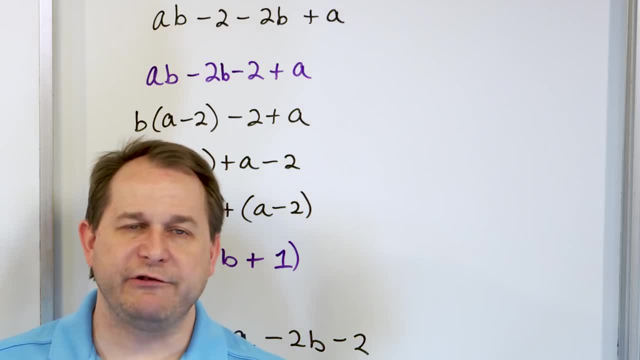 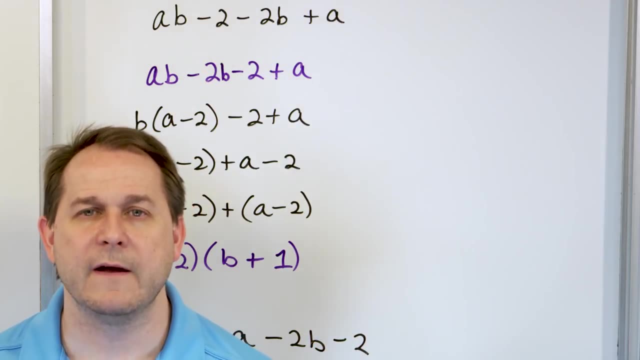 factoring general trinomials, And it's just going to be an incremental, step-by-step type of deal. We'll rebuild our skills, But ultimately, what we're going to do is learn how to factor all these kinds of expressions so that we can then factor out the things that we need to factor out. 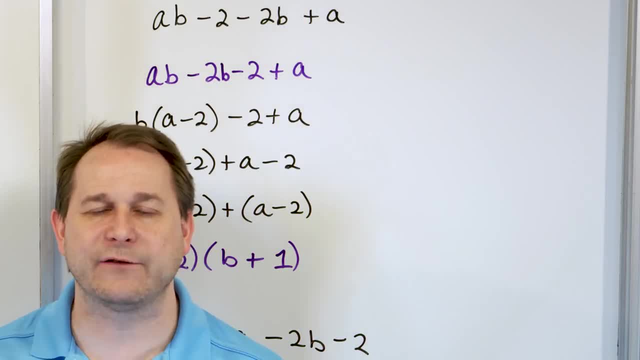 So we're going to solve equations that contain these kinds of expressions. That's why we're doing it. We're going to eventually have equations that'll look like: this equals something, And you'll need to factor it in order to be able to find the solution. That's why we're doing this. 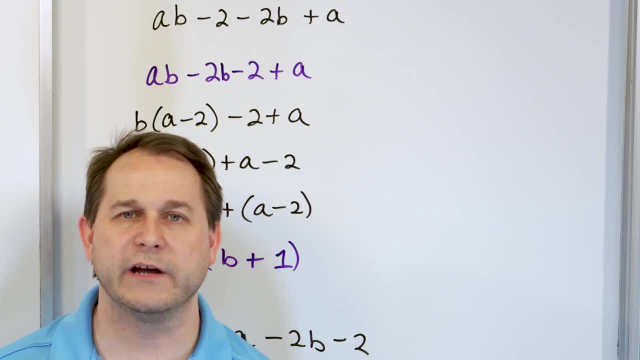 So practice your skills here. Follow me on to the next lesson. We'll continue working on this right now. 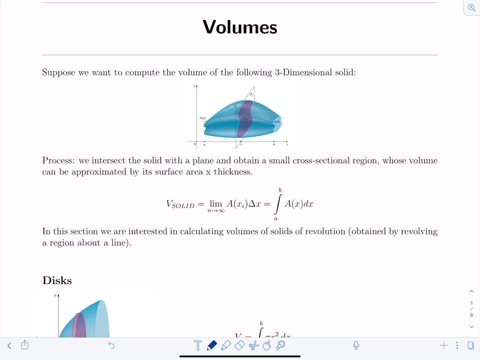 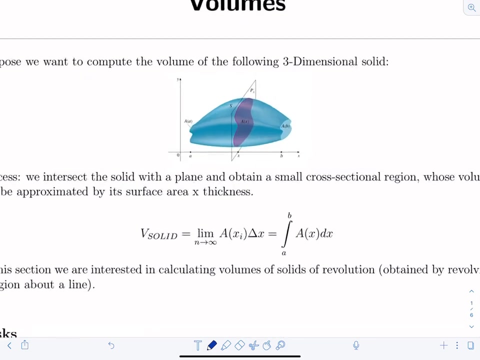 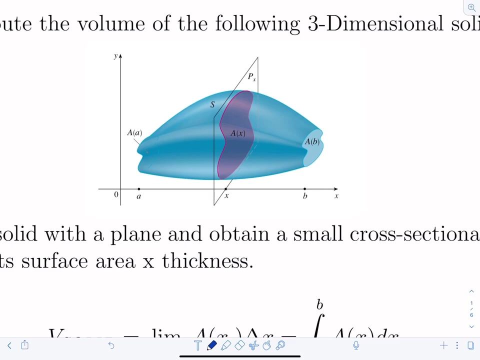 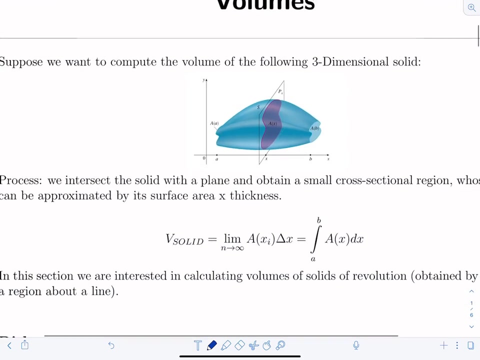 All right, so in this video we're going to change gears a little bit and start studying how to compute volumes using calculus. So say for example we wanted to compute the volume of the following three-dimensional solid. Up until now we've computed areas under curves but we can kind of take that process and extend it to find volumes of solids. So what's the process? Well, we intersect the solid with a plane and we obtain a small cross-sectional region, so a slice of the solid basically. Imagine like a bread slicer. And we can approximate the volume by taking the surface area of that slice, a of x, and multiply by the thickness of the slice. So I'm going to zoom in right now. a of x is the area of that slice, so that would be a two-dimensional quantity. And then the thickness of the slice would give us a our third dimension. Okay? And as you can imagine, the more slices you take, the better approximation you have for the volume of the solid. So that's why we say that the volume of the solid is equal to the limit as n approaches infinity as you take infinitely many cross-sectional slices of the area of x sub i. So that's the i-th subinterval where you're taking a cross-section times delta x, that's the thickness of the slice. And we've seen this expression before when we we're looking at the limit of our Riemann sum. And so we can write this as the integral, 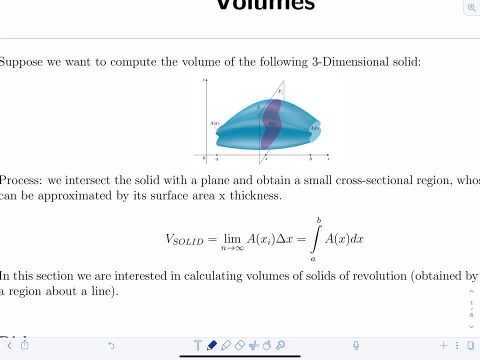 the definite integral from A to B, as long as the solid is bounded from between A and B, of A of x dx. Okay, so if you're integrating an area, then the result is going to be a volume. 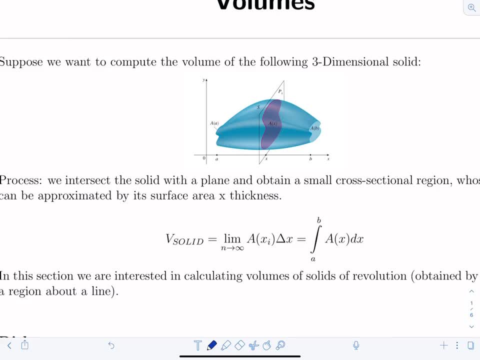 Basically, the dimension will always increase by one because A of x is two-dimensional quantity, 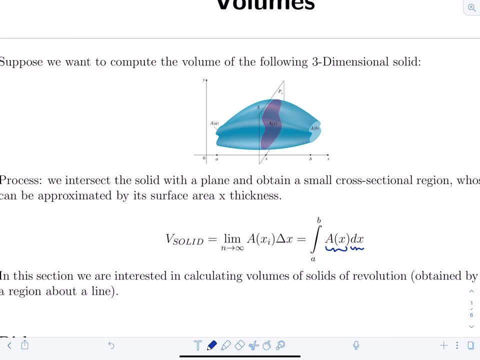 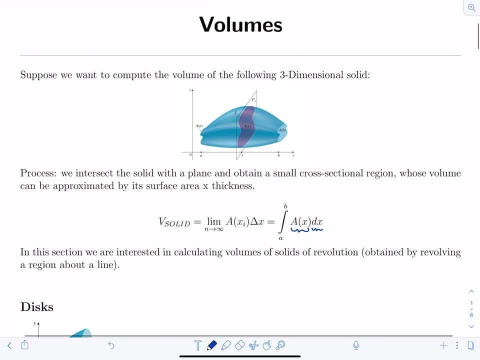 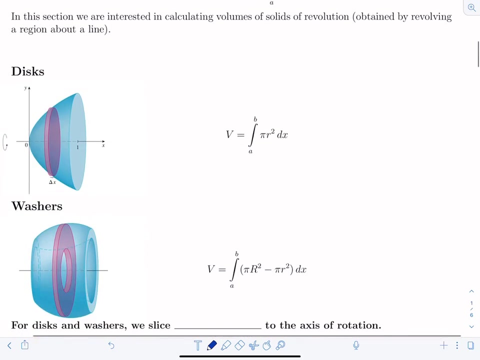 and then dx basically adds that third dimension. Okay, so in this section, we're going to look at a very special kind of solid, a solid of revolution. Well, what is that? It's obtained by taking a region and revolving or spinning it around a line. So this is a very specific kind of solid that we're going to focus on for the time being. And the process that we're going to look at in this section will involve either using disks or washers. So I'll explain what that 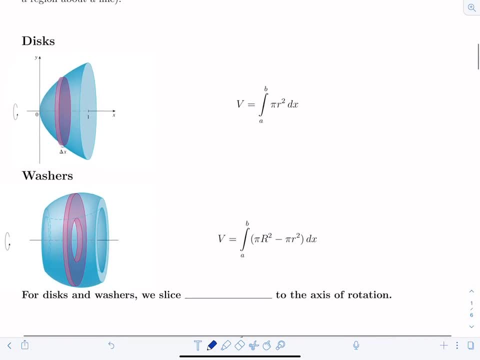 is. So when you take some region and you will revolve it, let's just say around the x-axis,